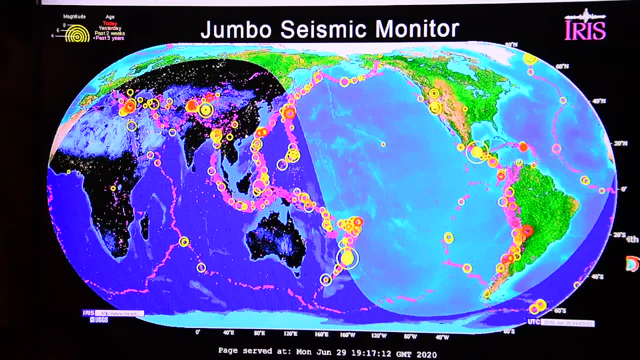 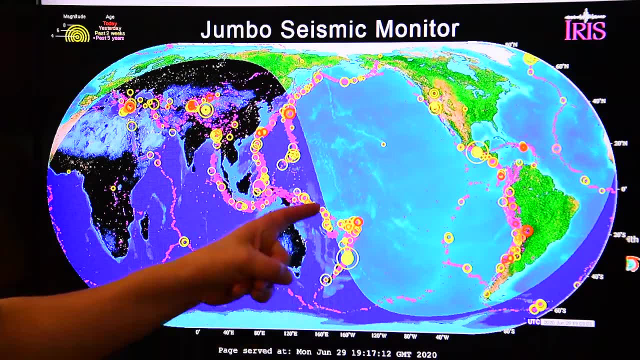 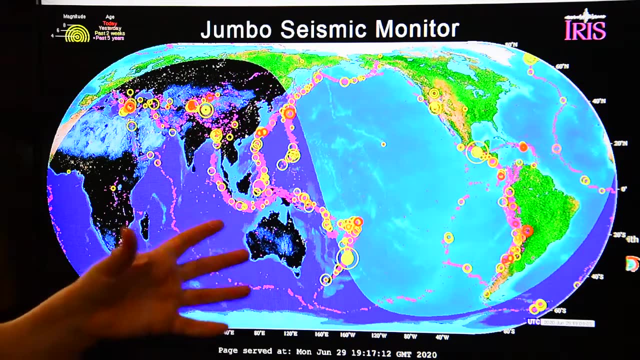 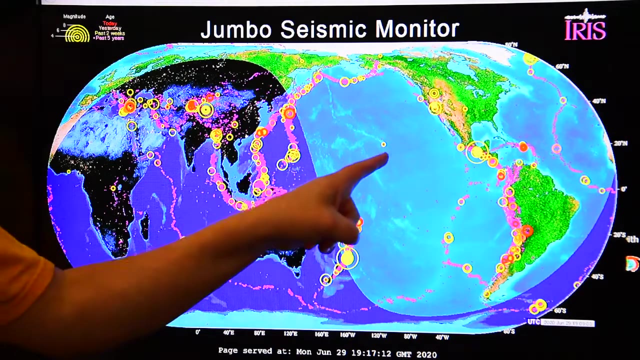 day- and this is kind of a typical day- of earthquakes, and what you hopefully will notice is that earthquakes tend to happen in specific locations. they're not scattered around the entire planet. in fact, they are mostly along plate boundaries. now, there are some exceptions, like that is Hawaii in the middle of the. 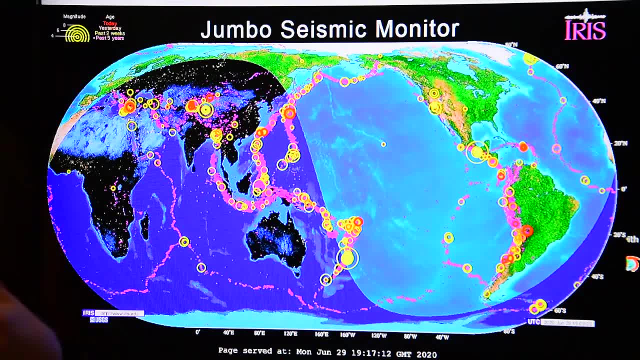 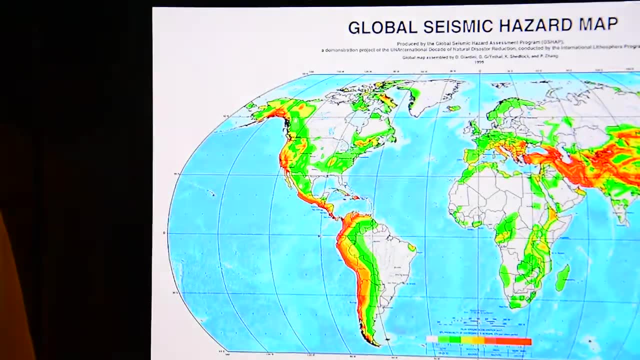 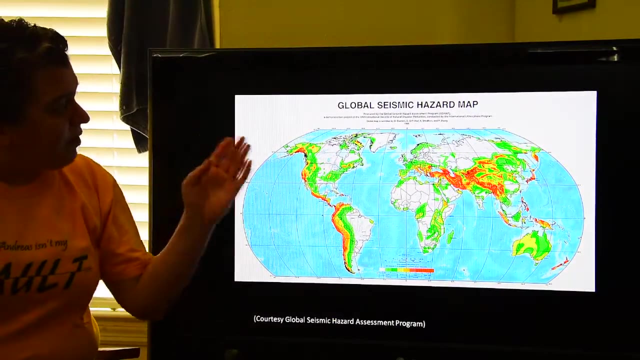 Pacific plate, but there's a volcano there, and volcanoes can also trigger earthquakes, and so, anyway, a typical day of earthquakes. now, the last thing we looked at was the earthquakes that have happened in the past few days. this is a seismic hazard map, and the darker reds are places where 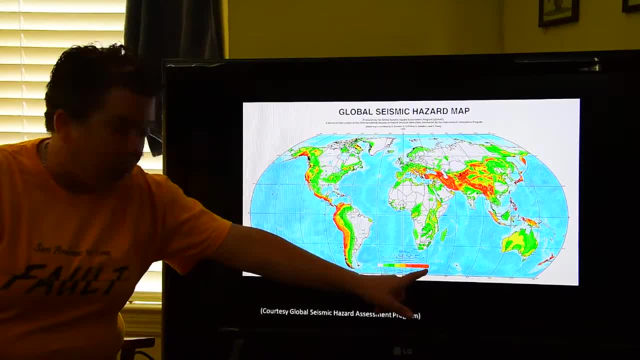 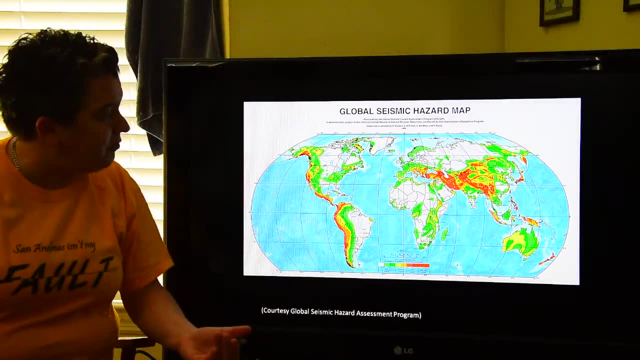 you can see the ocean, and the ocean is a little bit darker and you can see the where you have a greater chance of earthquakes happening. and then, as we go this way, to like the yellows, the green and white is where there's less of a chance. so here in Texas you can see it's white there. that doesn't mean that we 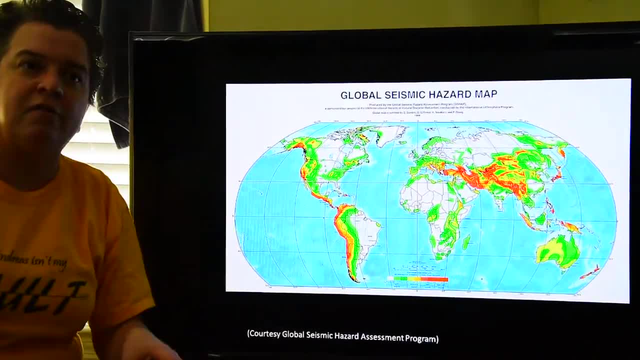 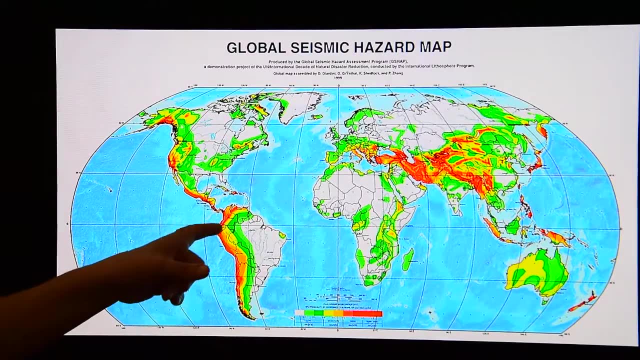 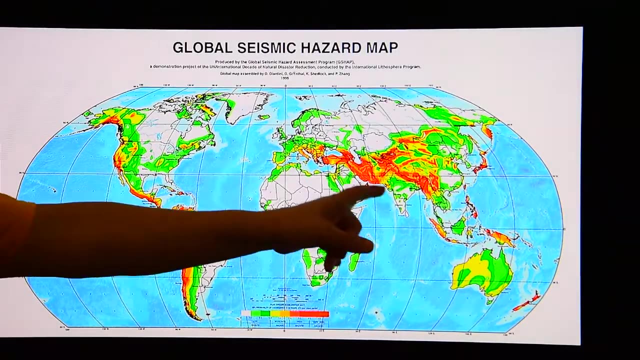 can't have earthquakes here. it just means that there is a much lower probability, a lower chance of earthquakes happening here than, say, in any of these places that are in red. and again, if we look at the bottom of the map and we look at this, the hazard areas correspond with plate boundaries. but 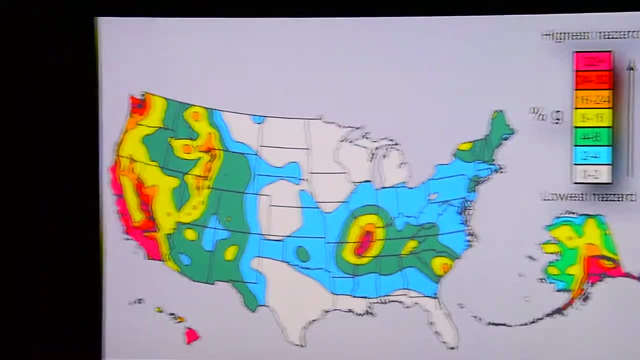 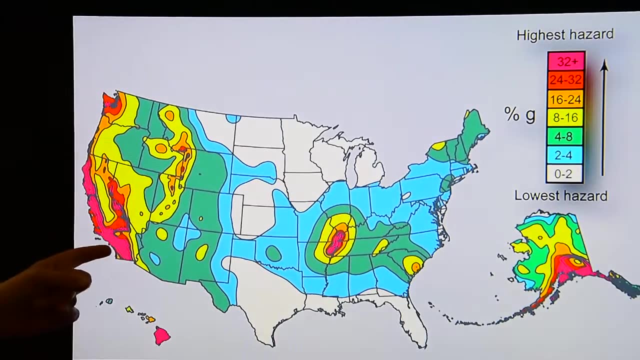 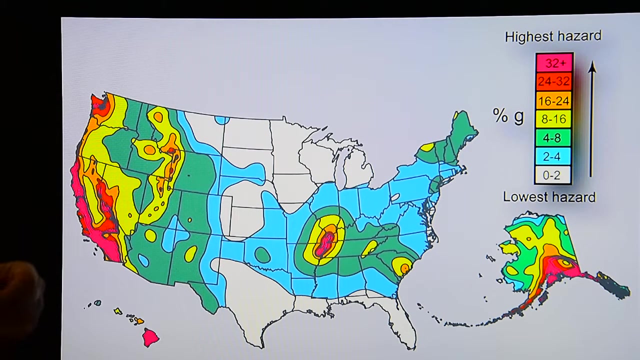 let's zoom in on the United States. here is hazard map for the US. again, red is the most hazardous, white is the least and you'll see plate boundaries, like on the western United States is the highest hazard. but a few places stand out. we can see here in South Carolina and here in the Mississippi Valley. 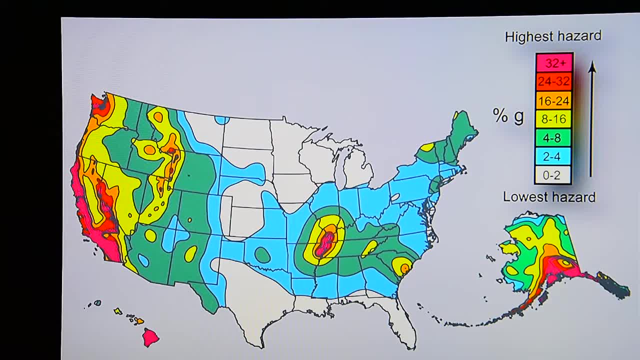 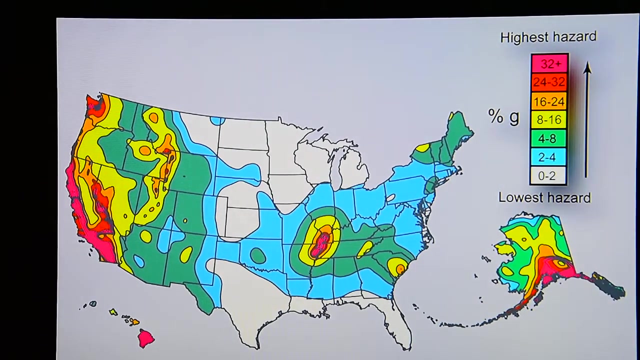 are places that are in the middle of the North American continent, yet they also have a higher probability of earthquakes, and these are called intra plate earthquakes, meaning within the plate, and the reason they can happen is these are not plate boundaries today, but in the past these were places where we had 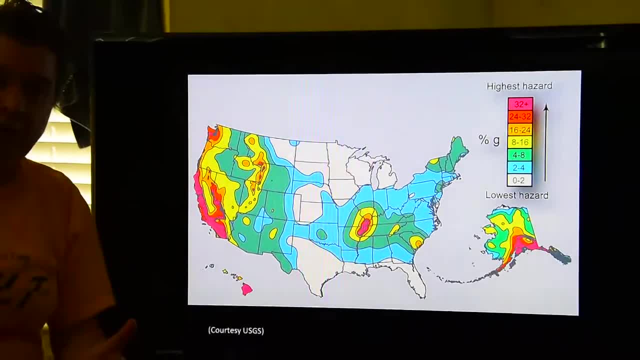 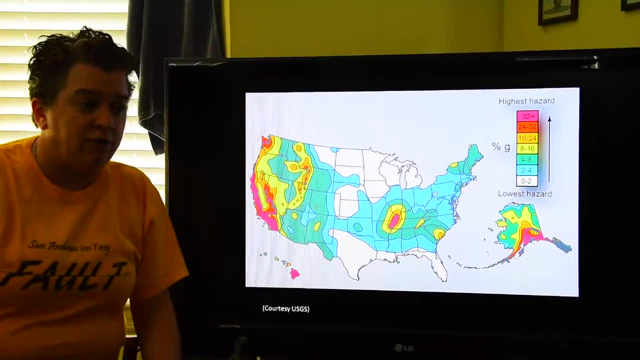 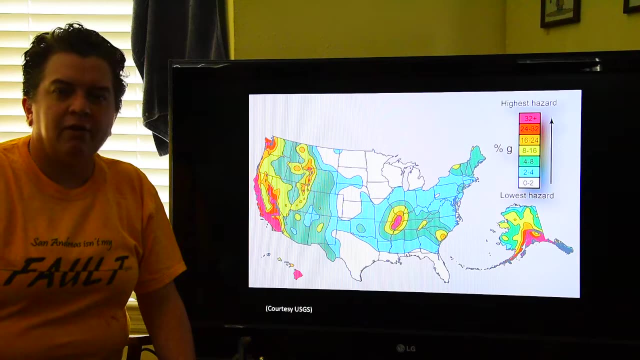 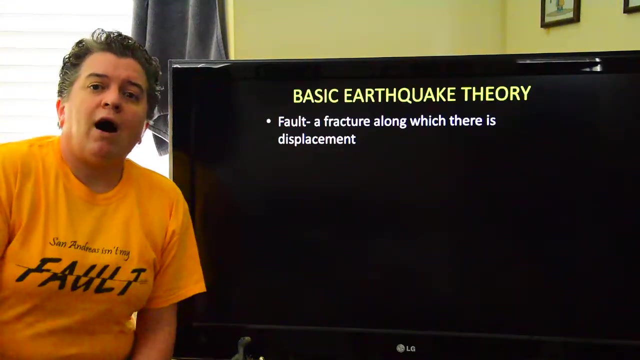 either plate boundaries or tectonic activity, and there are still some locations where they still happen as bad, so you still can have a chance of earthquakes happening in those locations. Joe, don't eat that. sorry, my cat thinks anything that's on the floor is edible. all right. 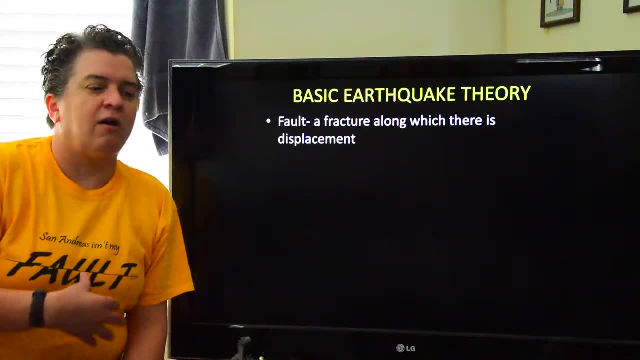 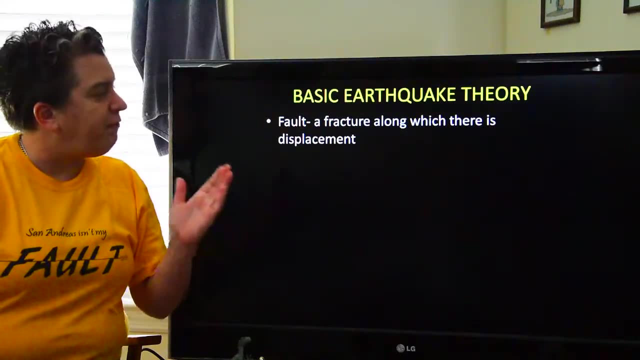 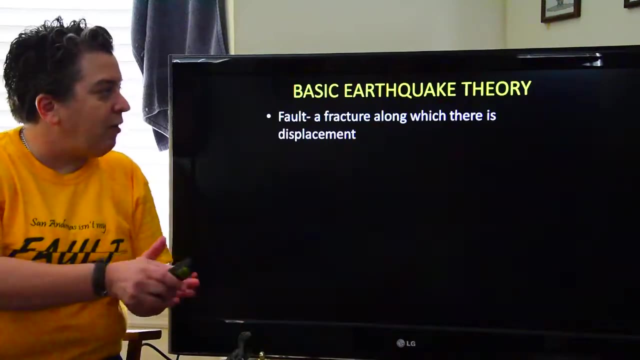 so let's talk a little bit about why earthquakes happen. now that we've seen them, places where earthquakes are likely to happen have these things that are called faults, and a fault is a fracture or basically a crack in the planet or the rocks where there's movement. okay, so if you have a 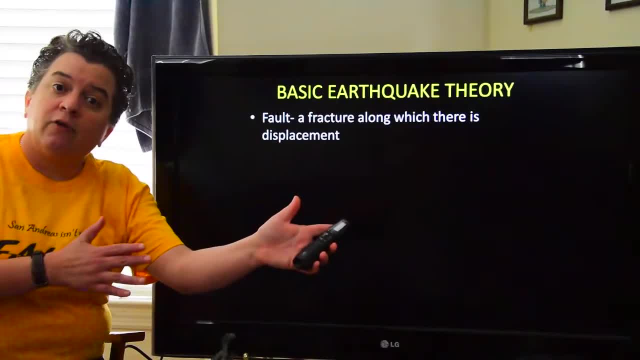 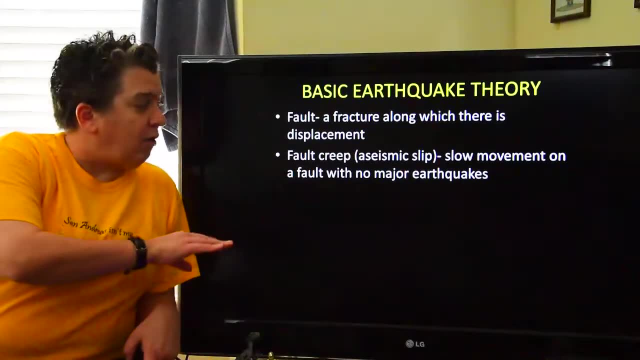 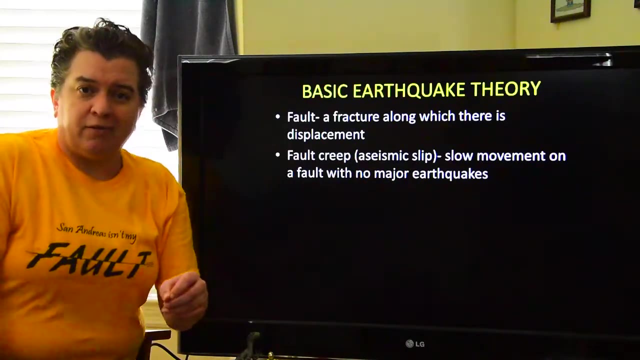 fault. the rocks on one side of this crack are moving relative to the rocks on the other side. now, where you have faults, you can have something called fault creep, which is also called a seismic slip. okay, so a little bit about science. in science, lots of our words have either Greek or Latin root words. 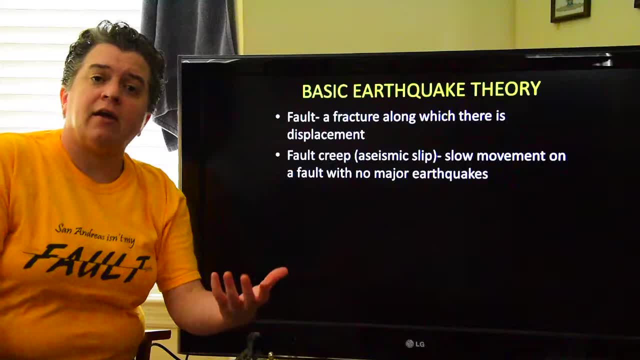 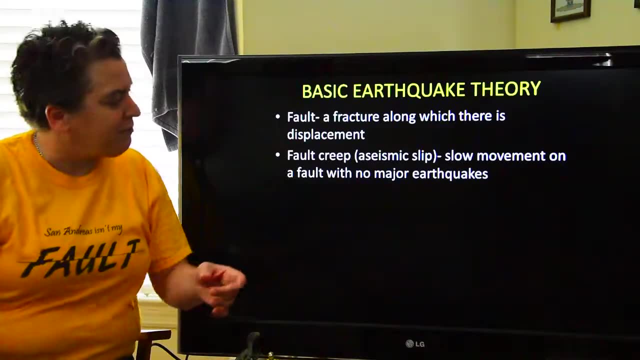 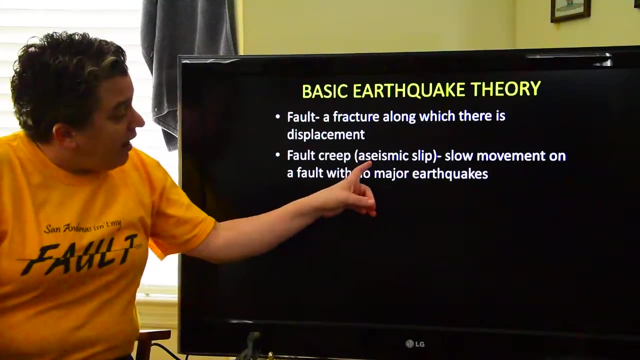 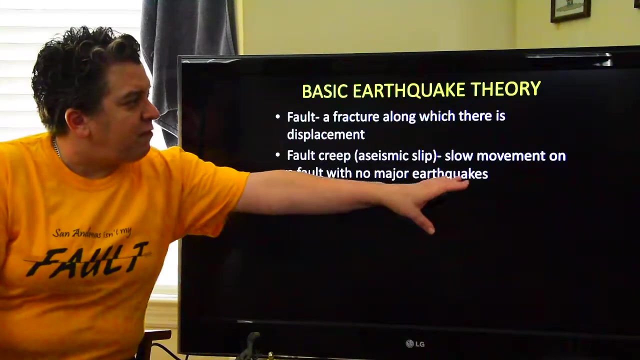 seismic. seismic means shaking in Greek, so anytime you see something to do with seismic, it's referring to shaking earthquakes. so a seismic- now the prefix a in Greek means not, so if we have a seismic slip, it means movement without shaking, and this is fault creep and this is where the rocks on either side of the 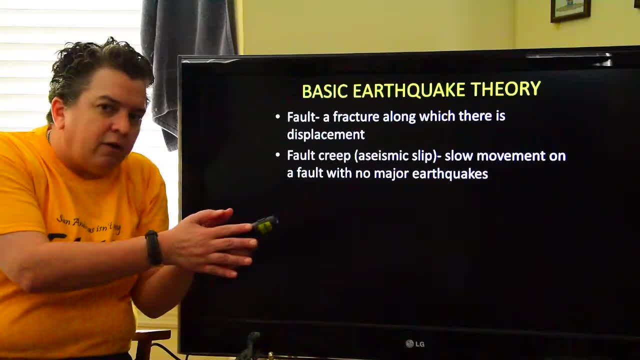 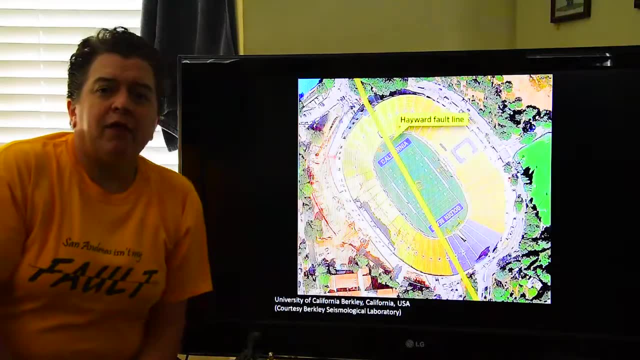 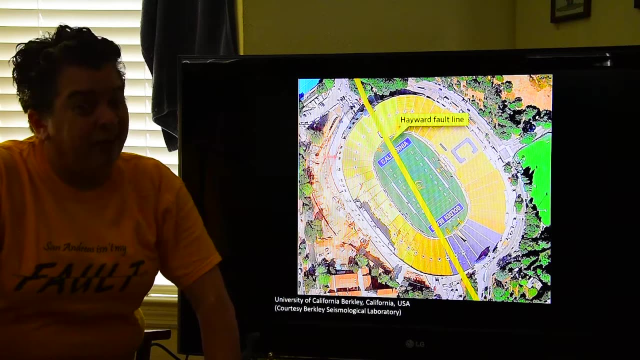 fault are just slowly moving alongside each other and so you have no major earthquakes occurring. and you might think, well, that's a good thing, right, if no major earthquakes occur, we don't have to worry about this. well, that's not exactly the case, and as an example of the fact that a seismic slip is still a 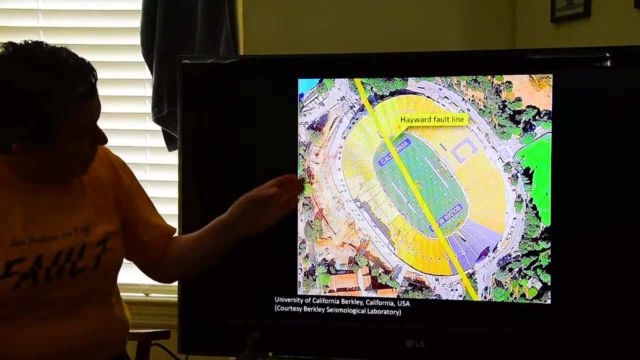 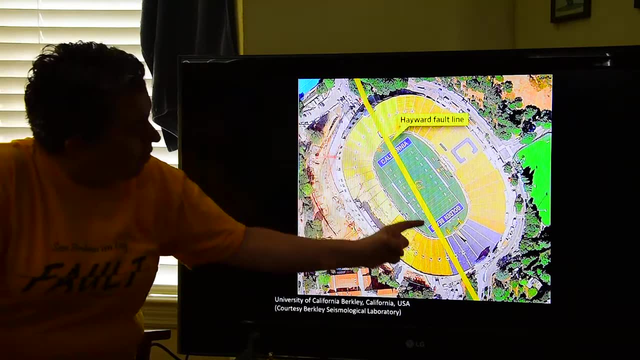 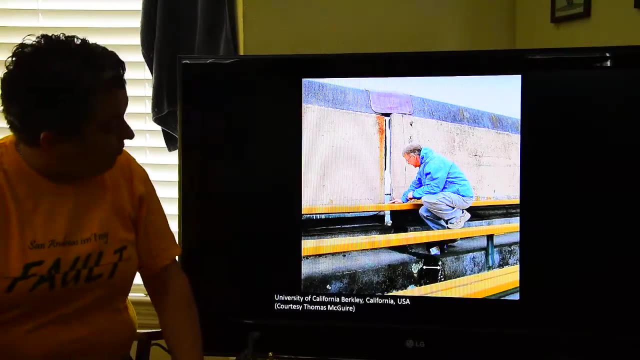 hazard that should be considered. let's take a look at the University of California Berkeley football stadium. it was built right on top of the Hayward fault line, so the next place we're gonna go we're gonna visit right inside the football stadium. do you notice how the 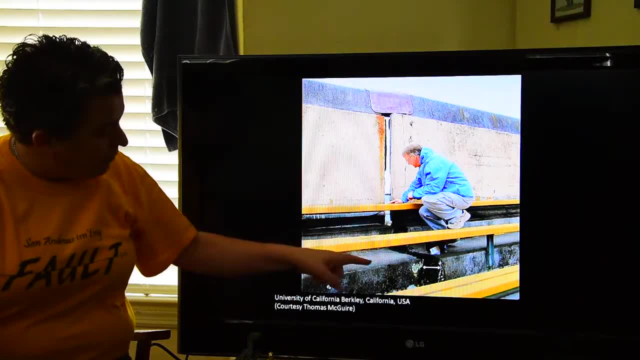 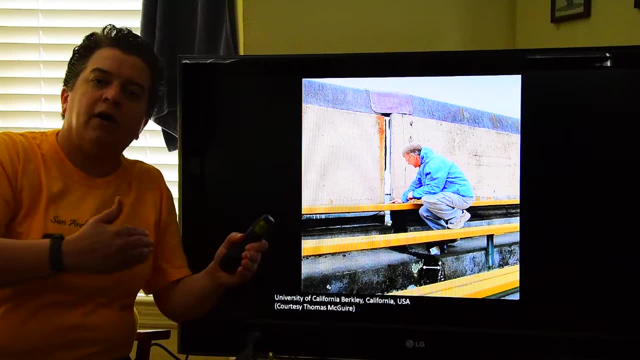 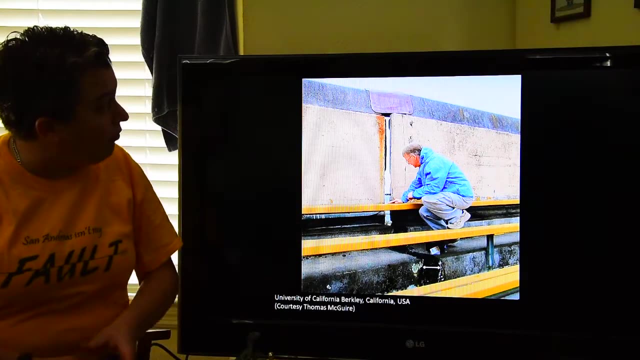 wall no longer matches up. right, it's actually moved and that's because the Hayward fault is slowly creeping along and over time one half of the wall is moved and over time the half of the stadium is still moving. ok, so the other half of the football stadium is headed in one direction and the other half is headed in the. 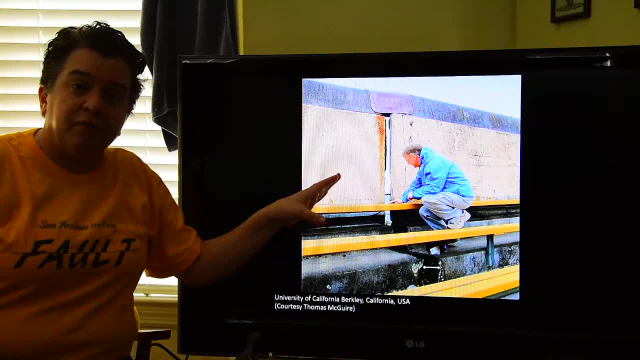 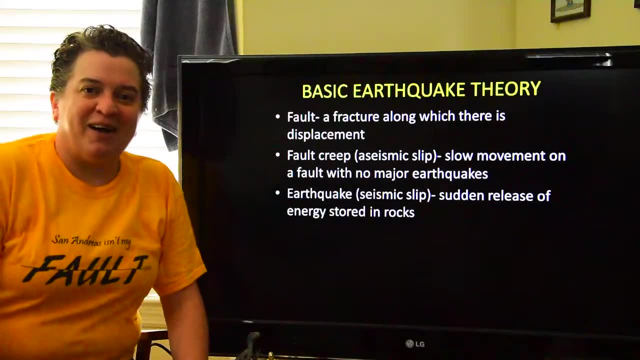 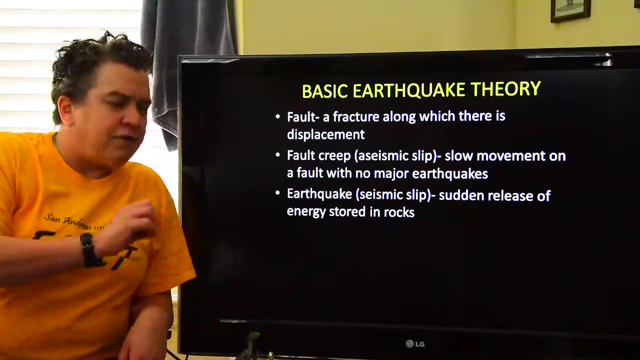 other direction, and so, even though there's- no, there haven't been any major earthquakes, it's still definitely something you need to consider. building on faults, now we also have what's called seismic slip. seismic slip is an earthquake. it's where we stored in rocks, So you might be sitting there thinking well. 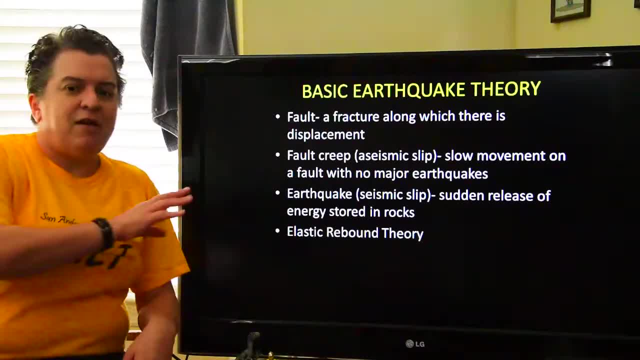 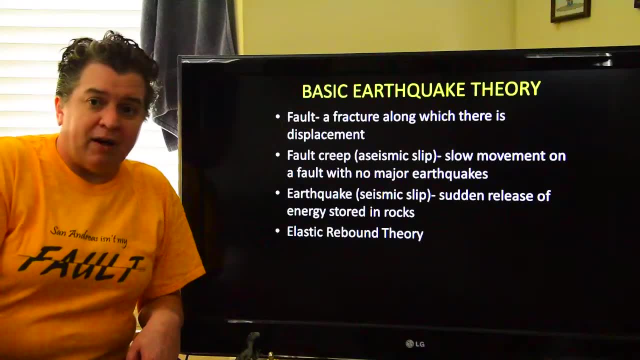 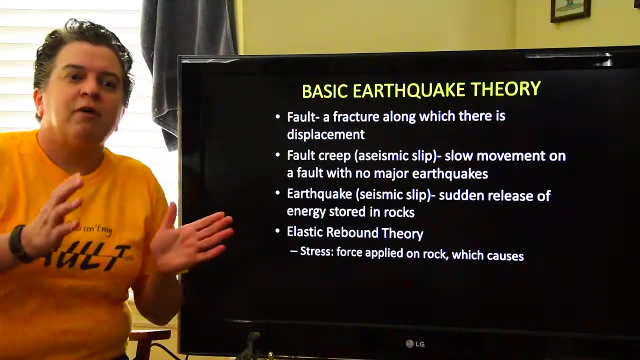 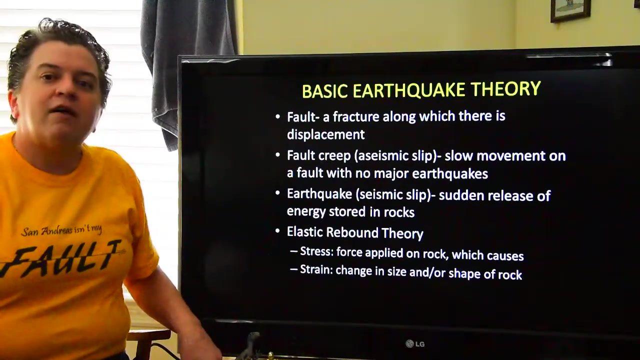 how does energy get stored in rocks? Well, this can be summarized in something called elastic rebound theory, And elastic rebound theory basically states that you have stress acting on a rock, some sort of pushing or pulling on the rocks. right, It's a force applied to the rock, and this causes what we call. 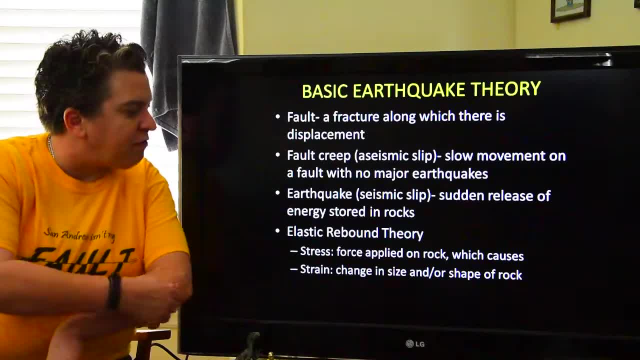 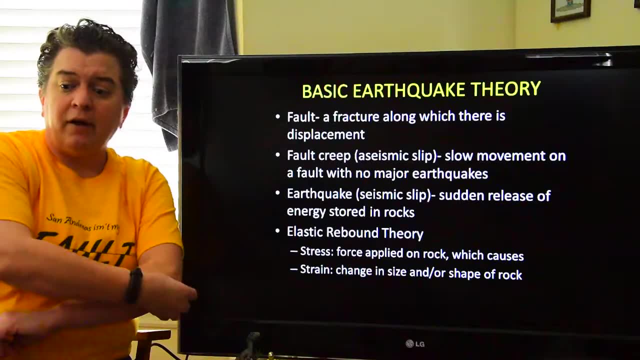 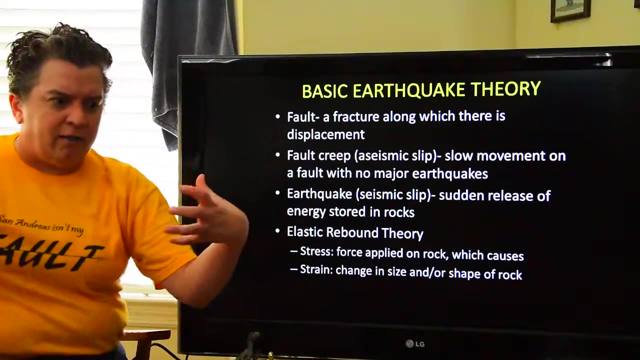 strain. Strain is a change in size and or shape of a rock And you can imagine elastic rebound theory, thinking of a rubber band. right, You can pull on the rubber band and it changes size and shape And then if you let go it kind of like you can shoot it across the room, right? 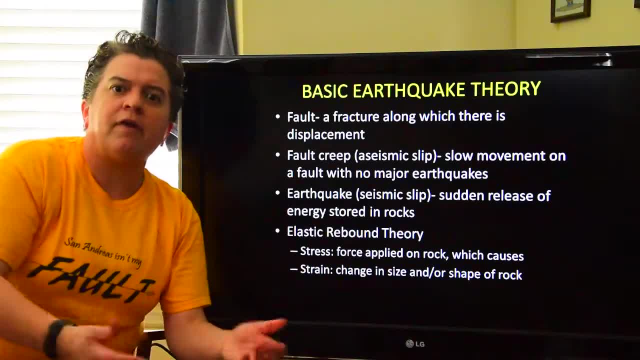 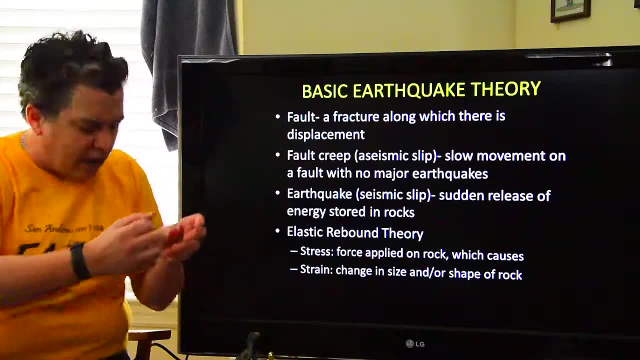 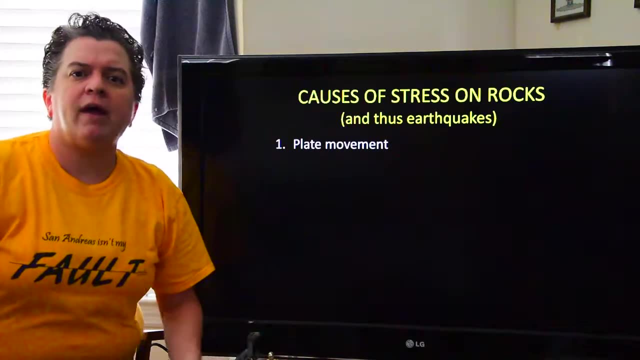 And that's the energy that was stored in there being released. The same thing happens to rocks. You have these forces applied to the rock. It changes the size and the shape of the rock, but eventually that gets released and the earthquake happens. Well, what causes stress on rocks? 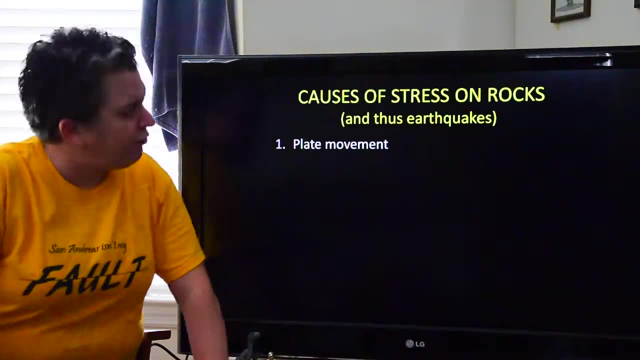 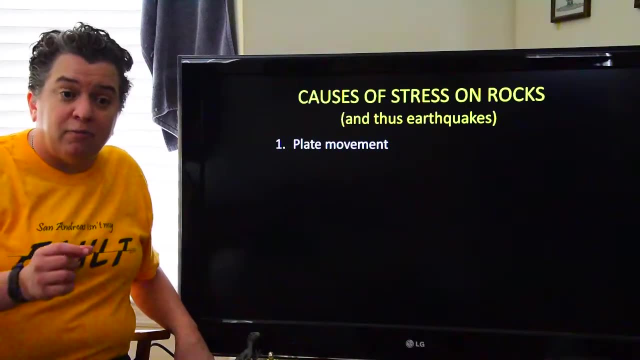 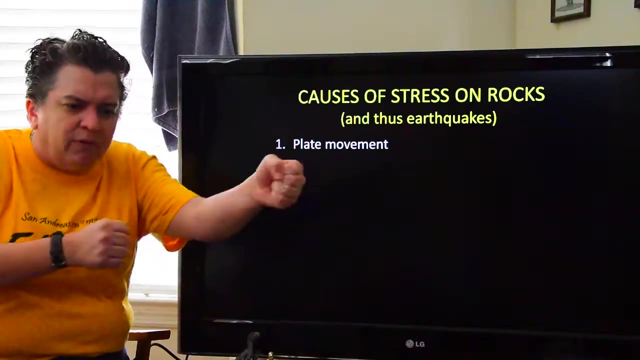 What forces get applied to rocks to cause that to occur? The biggest one is the movement of those tectonic plates. Last lecture I said plates are moving a few centimeters every year And as this movement happens it pushes on some rocks and pulls on. 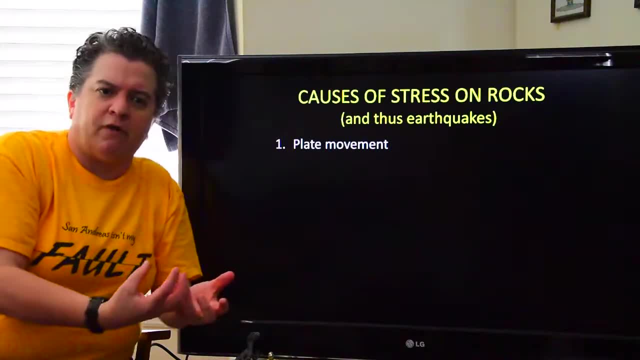 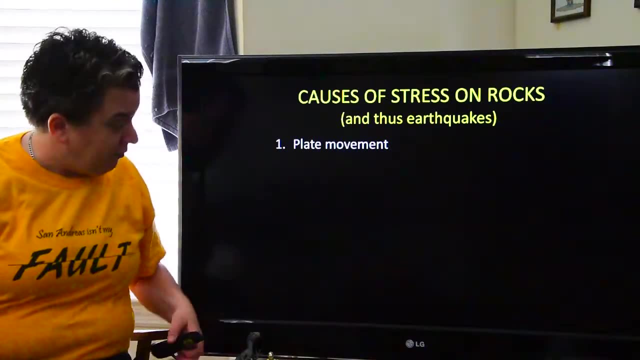 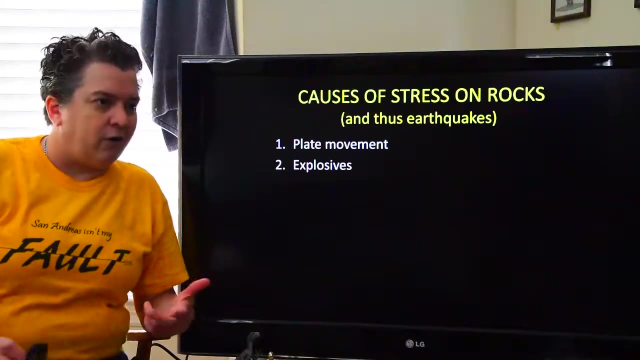 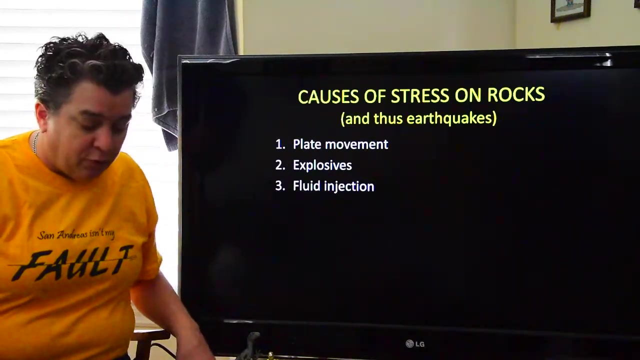 on others And this is exerting a force on those rocks And that's why most of the earthquakes we see are along plate boundaries. But there are other things that can cause earthquakes, like explosives. Large explosives can cause earthquakes to occur. Fluid injection can cause earthquakes. 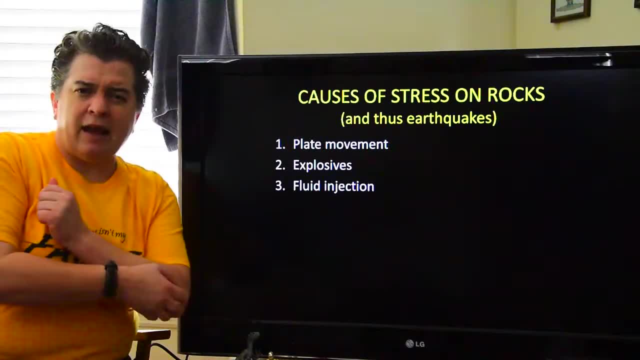 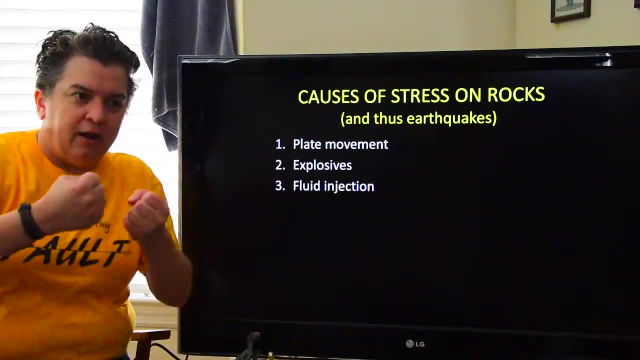 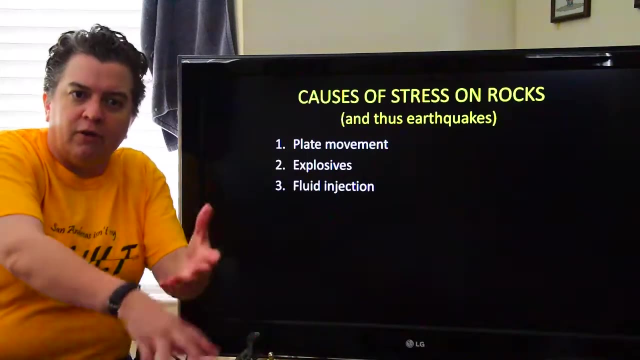 So a common way of getting rid of some really nasty, hazardous waste is to drill, basically, a well deep into the earth And then you inject, you force these nasty, toxic, hazardous fluids into the ground, you know, deep, deep underground. Well, I'm saying we're forcing it in, right? 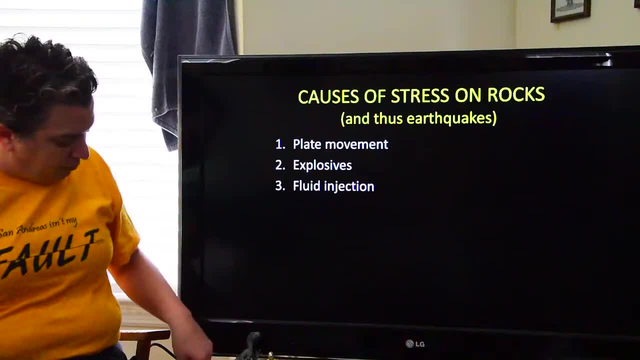 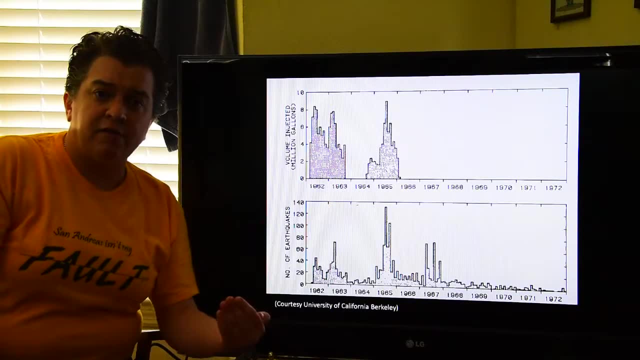 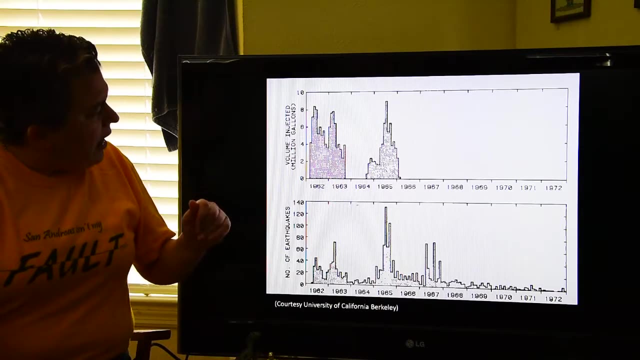 So that is going to be a force applied to the rocks, And we've seen in places where fluid injection causes higher seismicity, And the classic example of this is at Rocky Mountain, Arsenal, And here we have some records from the 1960s into the 1970s. 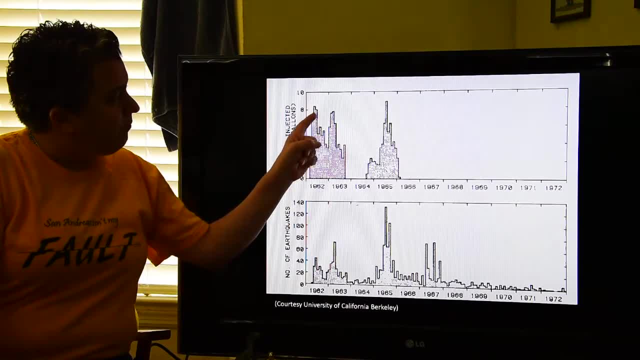 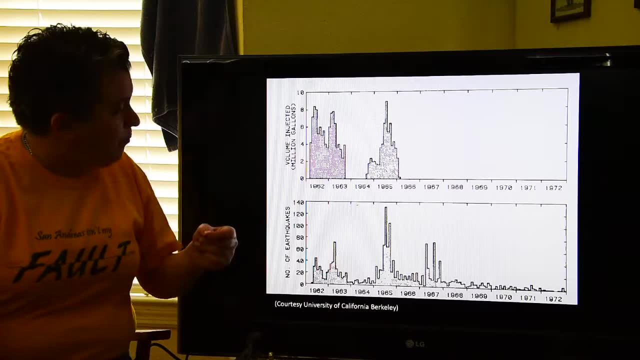 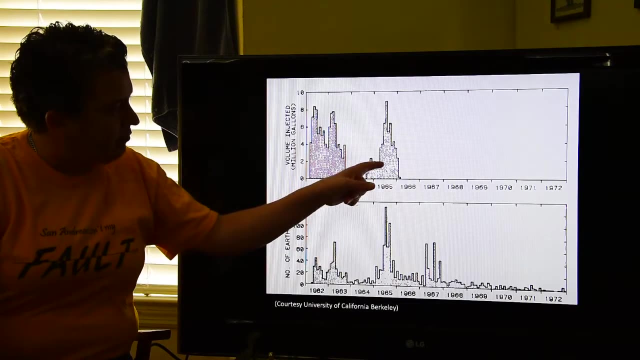 On this top graph we're showing the amount of fluid injected And then on this bottom graph we're showing the number of earthquakes that were happening, And you'll see when fluid got injected, more earthquakes occurred. When it wasn't injected, less earthquakes. 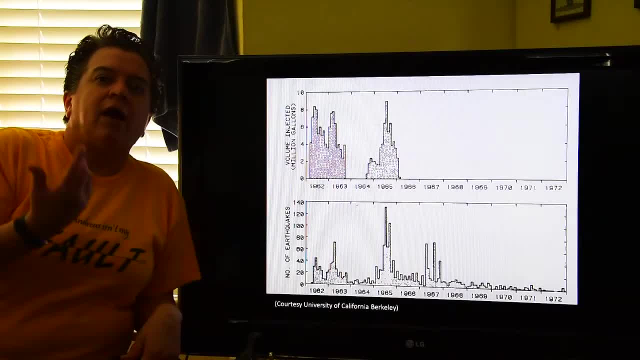 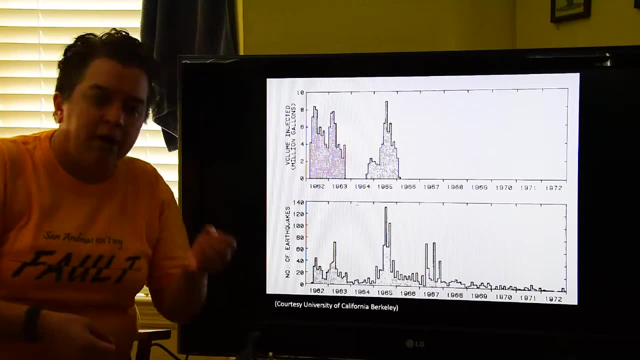 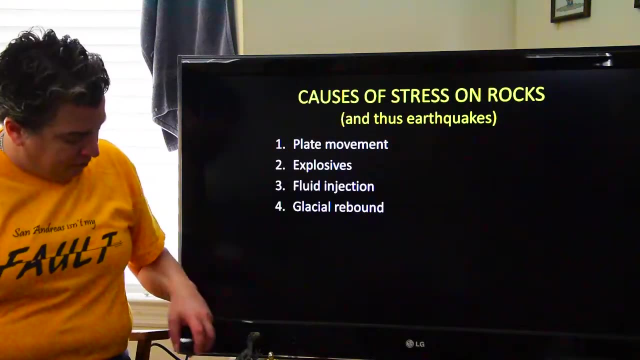 More injected, more earthquakes. And so what happens when these liquids are forced into the rocks underground? it exerts a force on the rocks and can make um earthquakes occur. Glacial rebound is another thing that can cause earthquakes. So glaciers are these big, thick masses of ice. 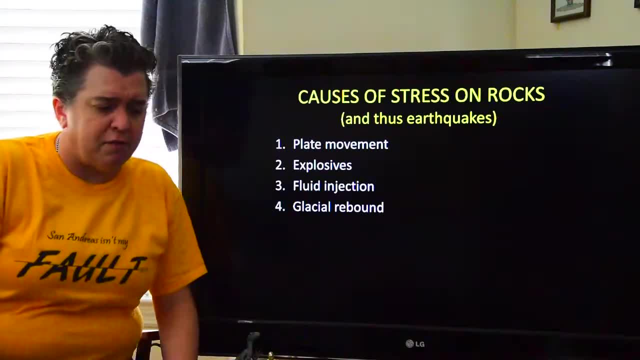 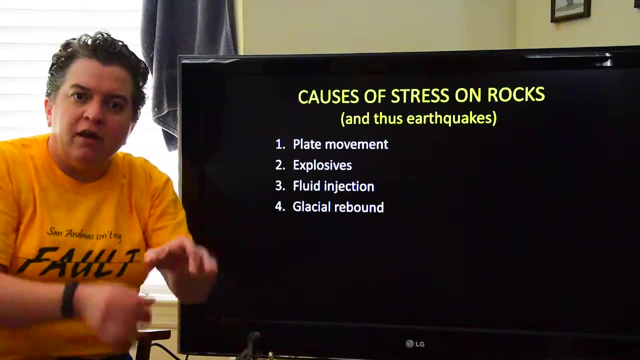 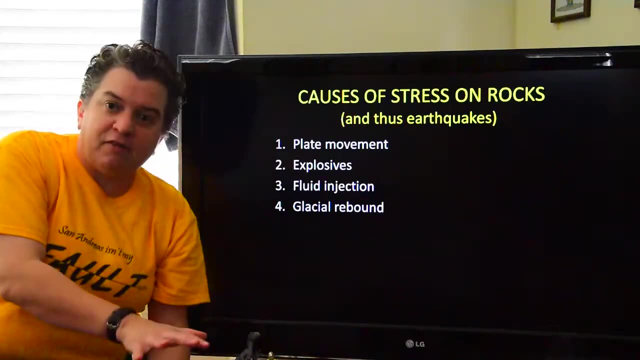 like three, four kilometers thick in some cases and that's going to weigh a lot. So you have this massive, massive weight on earth and that actually pushes the lithosphere down into that squishy plastic asthenosphere right. It actually sinks the crust downwards. 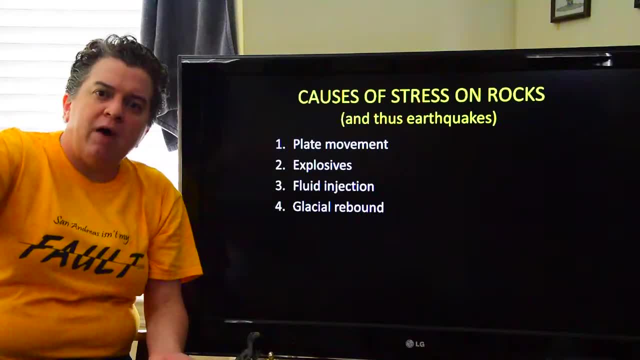 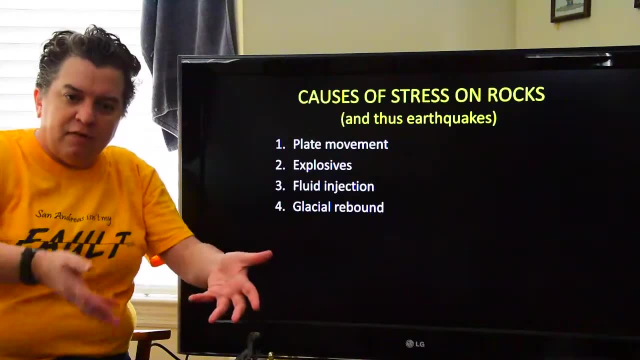 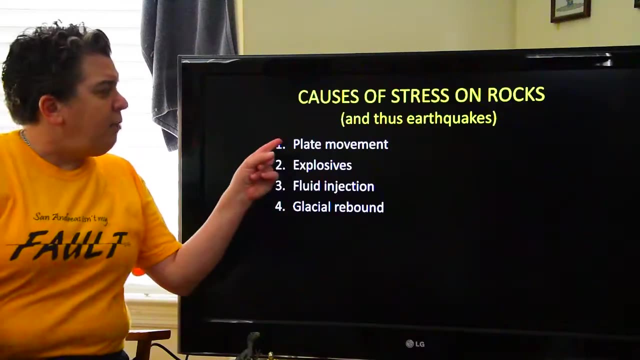 you can think. But when that glacier melts, there's no longer that weight pushing downwards, So the crust starts lifting back up And as that movement is occurring, that can cause earthquakes. So while the movement is increasing, the movement is increasing. 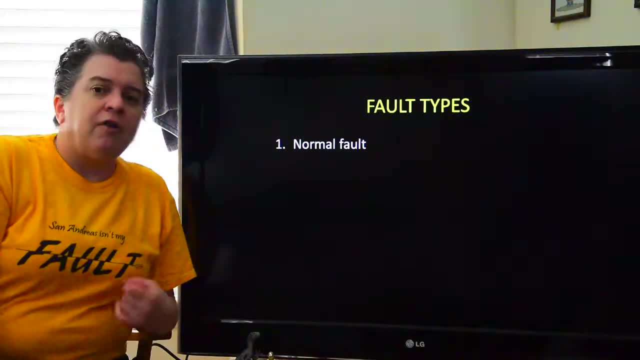 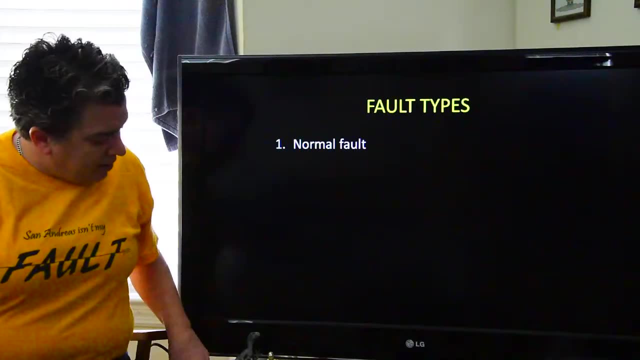 So, while the movement is increasing, the movement of tectonic plates might be the most common. Uh, there are other things that can cause earthquakes to occur. Now, we mentioned that earthquakes occur along faults. Faults are where rocks are moving right. 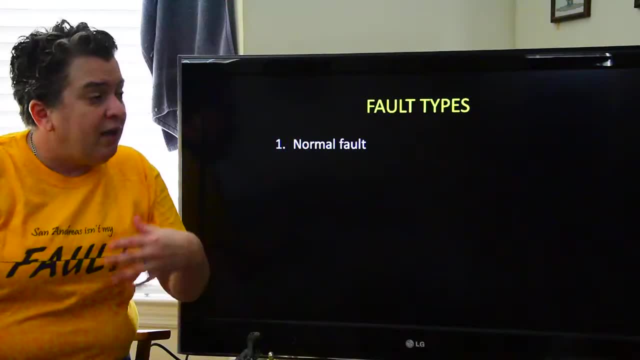 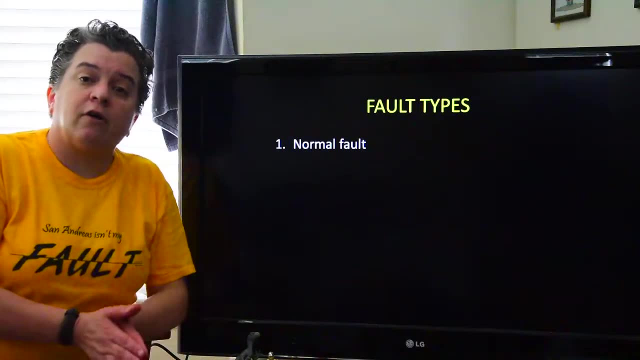 It's one of those cracks. Rocks are moving on either side. There are different sorts of faults that can occur. You have what's called a normal fault. This occurs at divergent plate boundaries, So that's where the plates are pulling apart from each other. And a normal fault looks like this. Right here is the fault, And see, this kind of purpley-gray layer of rock Matches up with that purpley-gray layer of rock That has moved down compared to this one. You can also have what are called reverse faults. 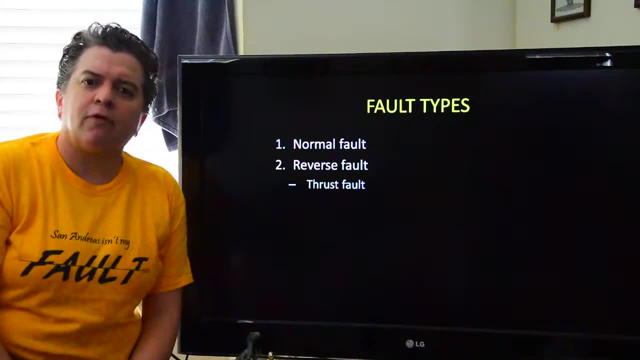 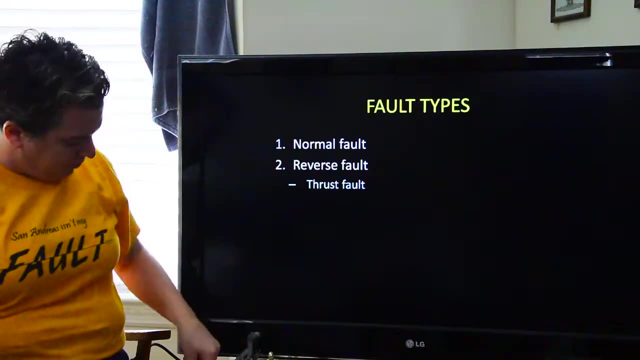 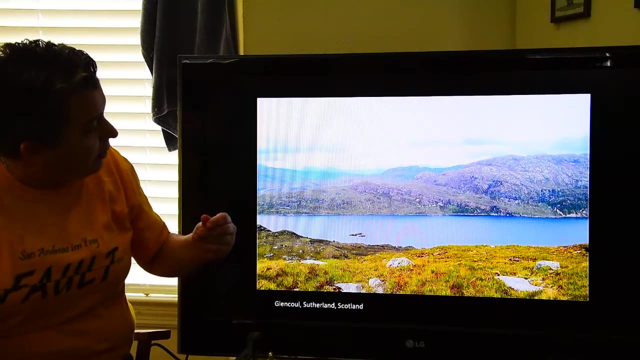 And probably the best known type of reverse fault is called a thrust fault. A thrust fault is a fault that moves up and down. A thrust fault is where rocks get shoved over top each other, And we can see that nicely here at the Glencoole thrust in Scotland. 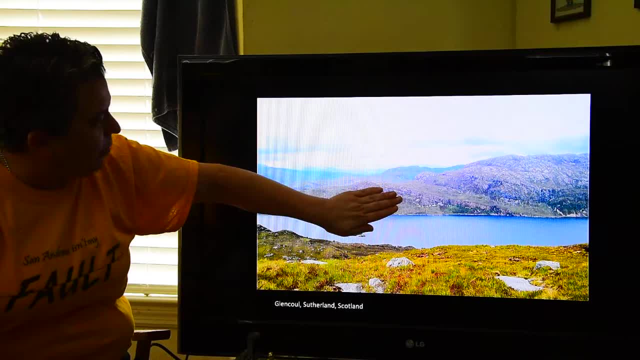 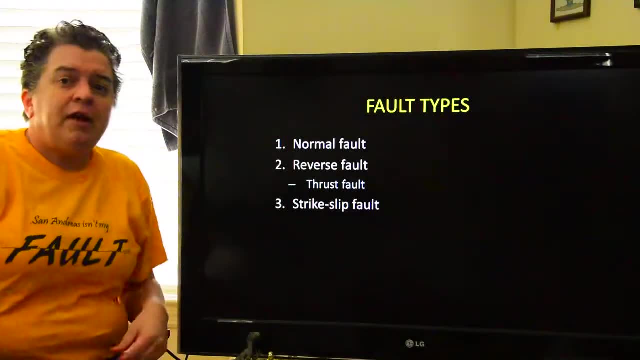 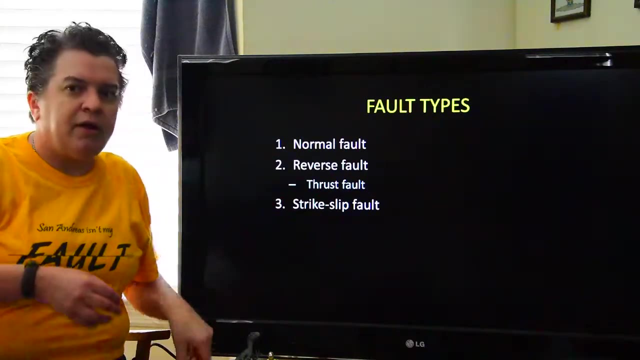 These rocks right here were pushed over top these rocks along a fault that sits right there. Then you can also have what are known as strike-slip faults And a strike-slip fault. the rocks are not being pulled apart, They're not moving. 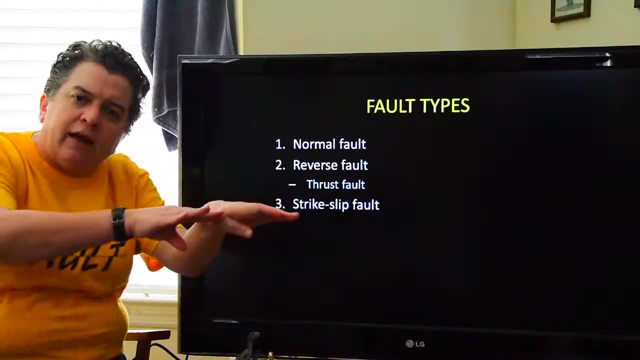 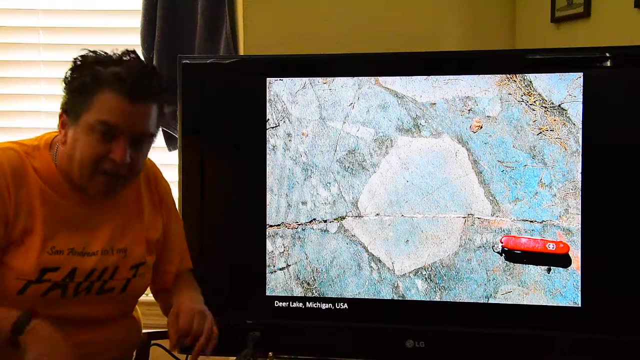 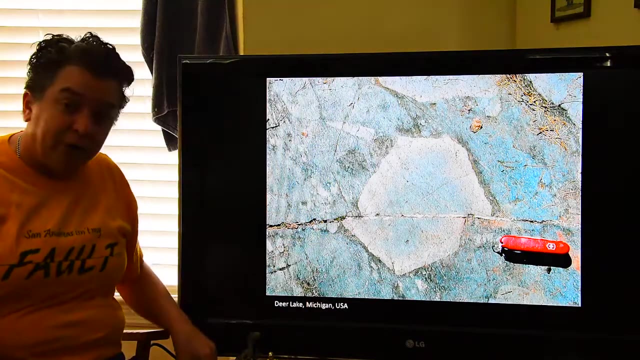 They're not moving. They're not being pulled apart or shoved together, They're just sliding alongside each other. We can see a very small strike-slip fault right here. We're looking down on this rock. You can see this side has moved just a little bit compared to this side down here. 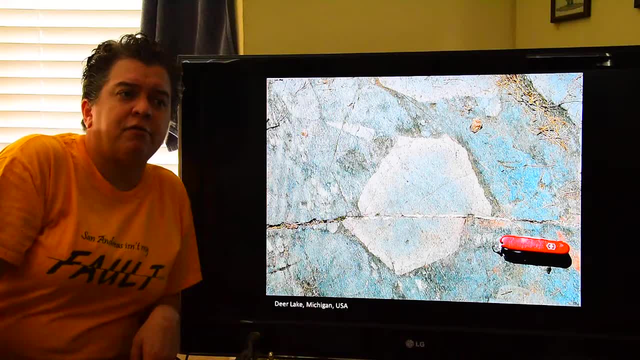 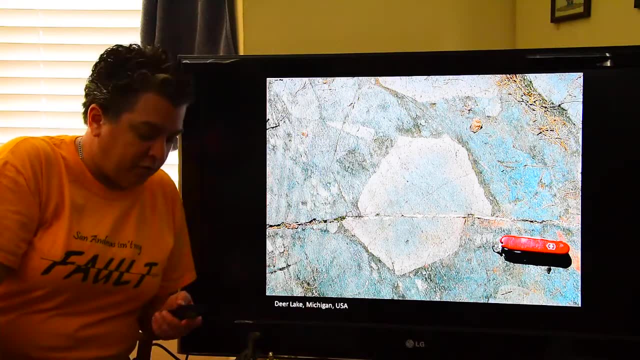 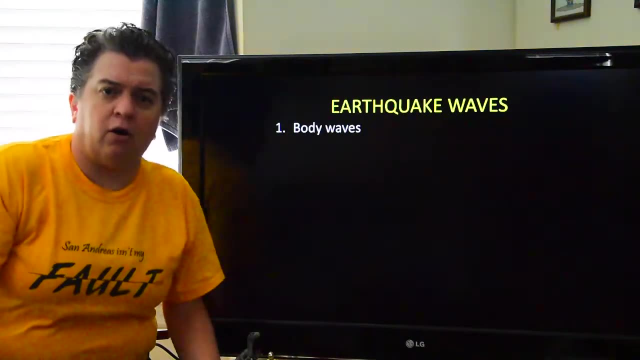 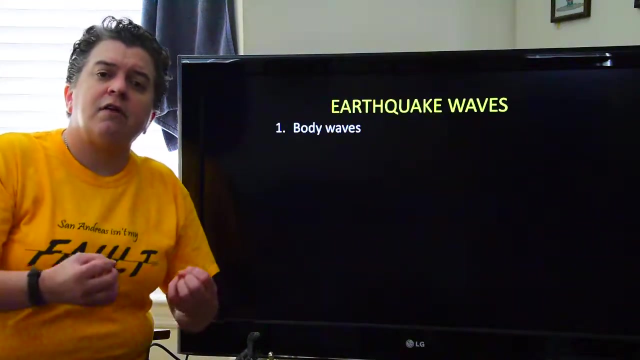 And those are your three basic types of faults. Typically, the earthquakes that are the strongest occur on thrust faults. Now, when an earthquake occurs, it's that energy gets released that was stored in the rocks, And the way the energy is released is in the form of waves, and that's the shaking. 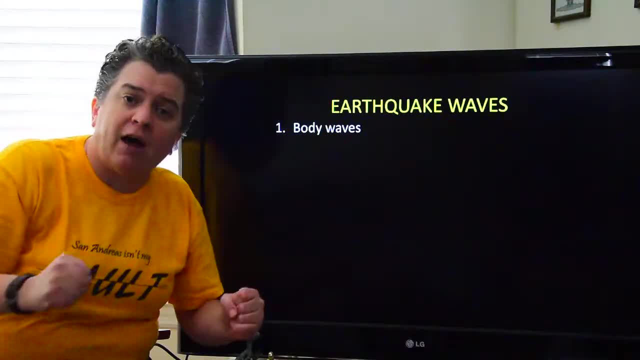 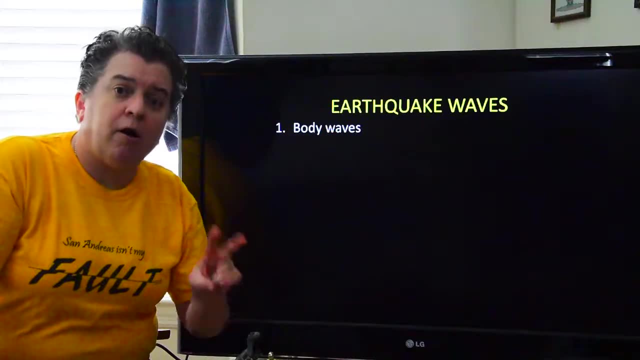 you feel. The shaking you feel is the earthquake waves traveling through the rock, And there are four basic types of earthquake waves. Two of them are called body waves and two of them are surface waves. So the first one is called the earthquake wave. 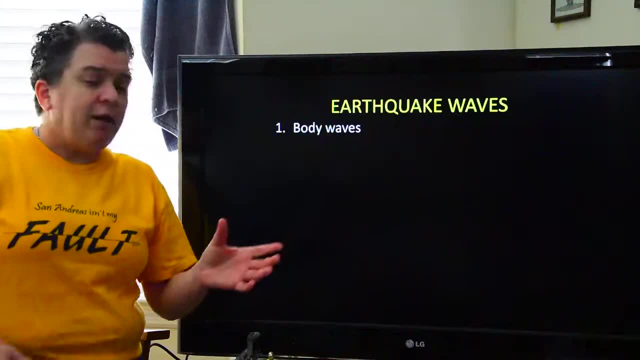 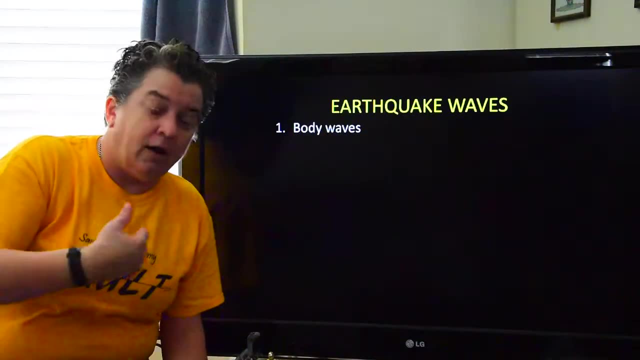 The second one is called the earthquake wave, The third one is called the earthquake wave And the fourth one is called the body wave. The body waves are called that because they will travel all the way through the middle of the earth and be recorded by instruments on the other side of the planet. 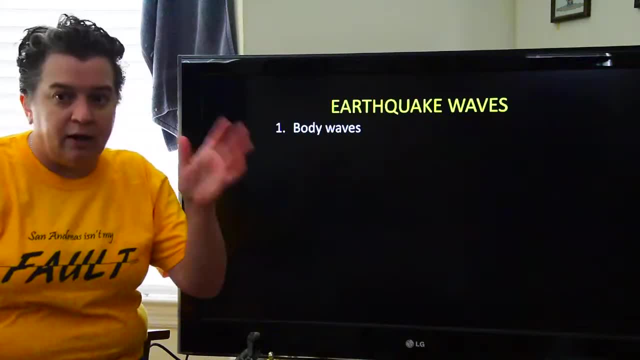 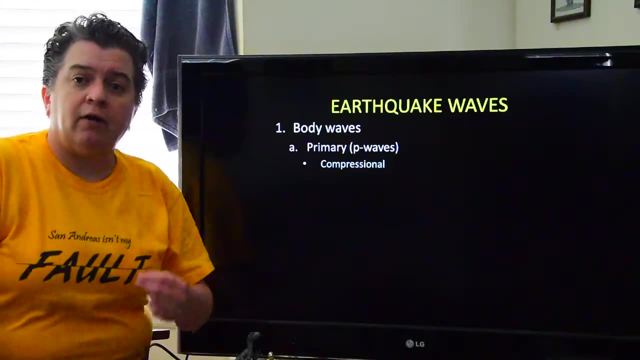 So these things will go through the mantle, they'll go through the core and out to the other side. And of the body waves one type are called the primary waves or P waves, And P waves have what's called a compressional wave. 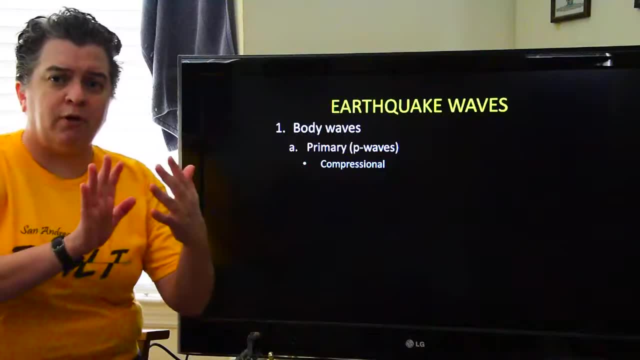 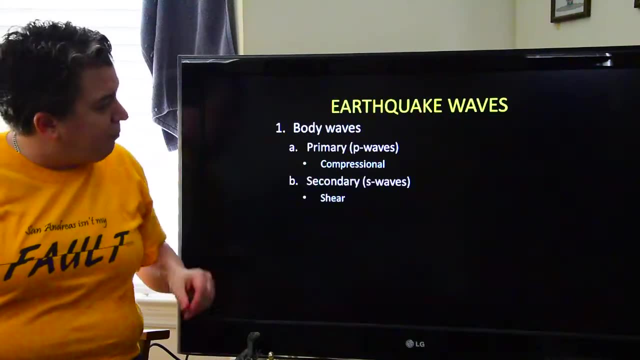 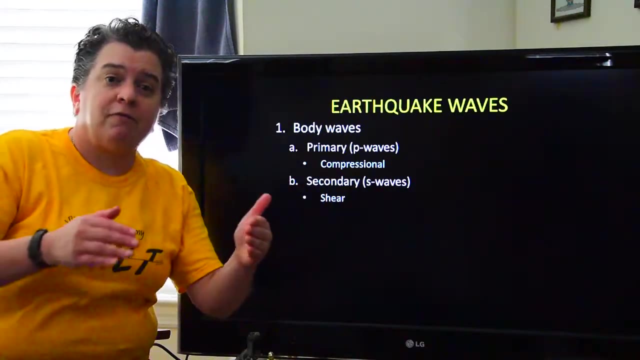 And the P waves are the primary waves. It's like a push-pull movement, So as they go through the earth they kind of squish stuff together and pull it apart. These are the primary waves because they travel the fastest and primary means first. 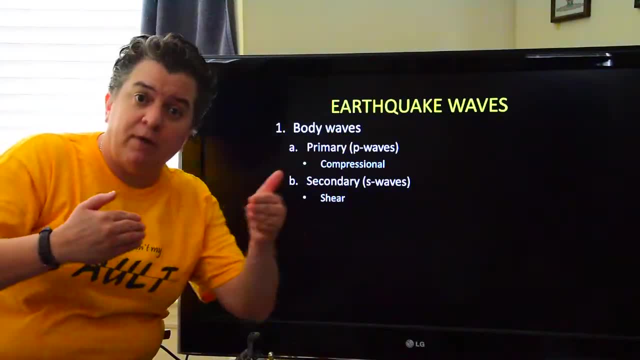 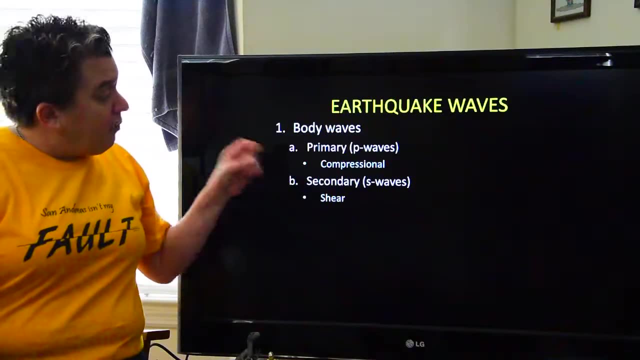 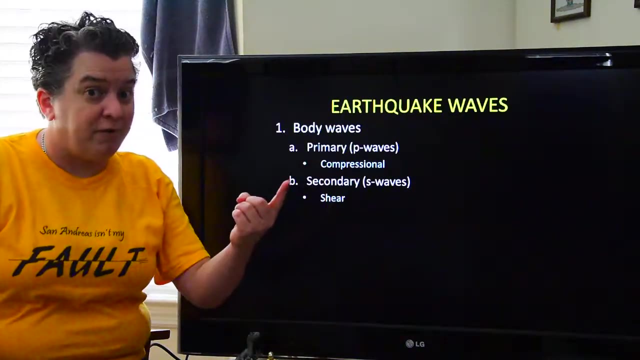 So, because they travel the fastest from where they begin, they're going to be the first earthquake waves that you can feel. So there's our primary waves, And then our other type of body waves are called secondary waves. Well, if primary are the first ones you feel, secondary are the second ones that you feel. 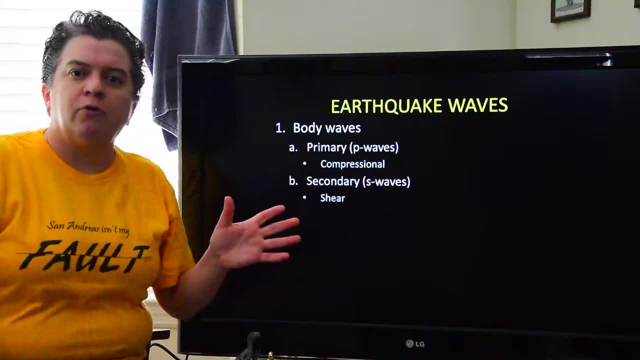 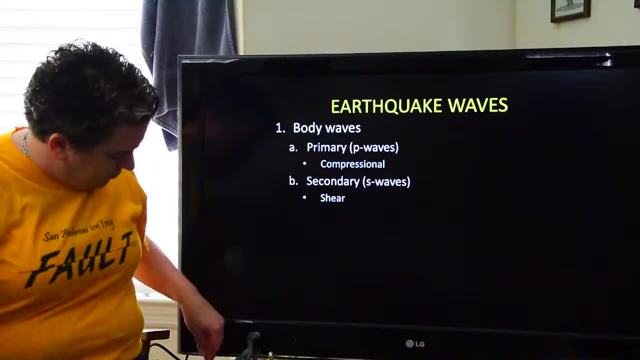 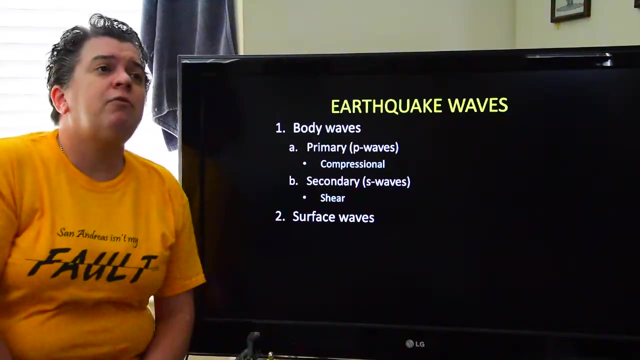 And we abbreviate it S waves, And these have a shear movement And shear is more like what you typically think of with a wave kind of a wavy motion. Now I also said there are what we call surface waves. Surface waves do not travel. 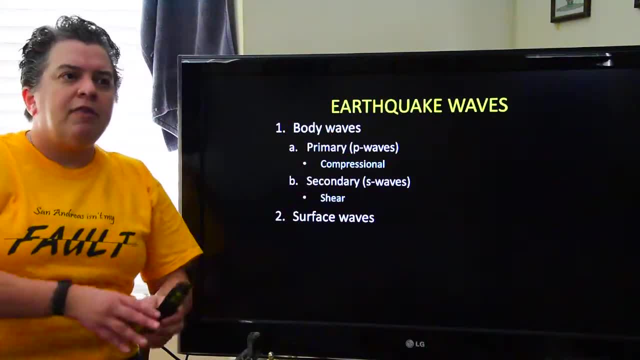 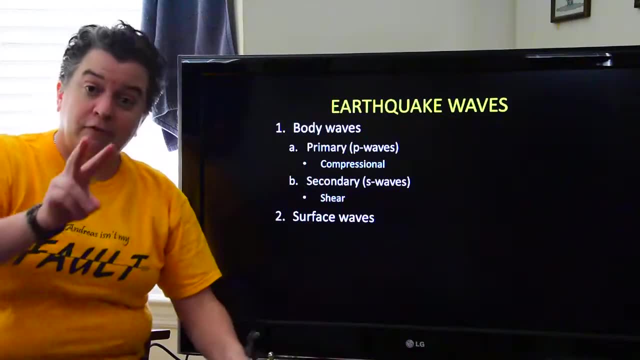 They don't move. They don't come to the interior of our planet. They travel around the planet by moving through the surface rocks. That's why they're called surface waves. There's two types of surface waves. We have the Rayleigh waves that move a lot like ocean waves. 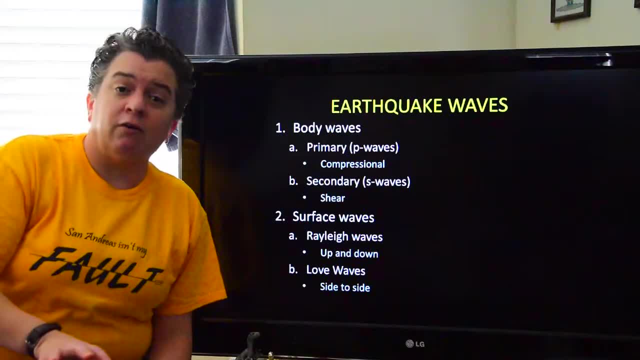 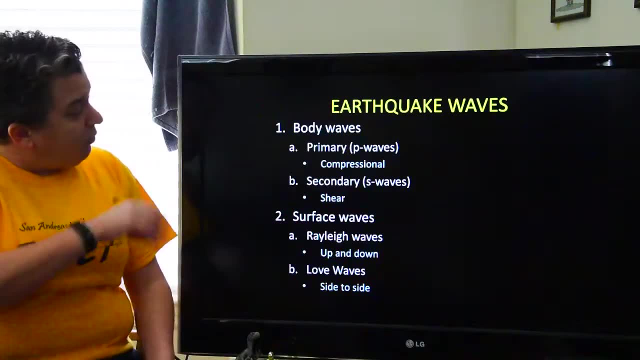 They're kind of an up and down motion, And then there's the Love waves, And Love waves- as they move forward, they're also kind of moving side to side. So when we have earthquakes, the primary waves are the ones that move the most. 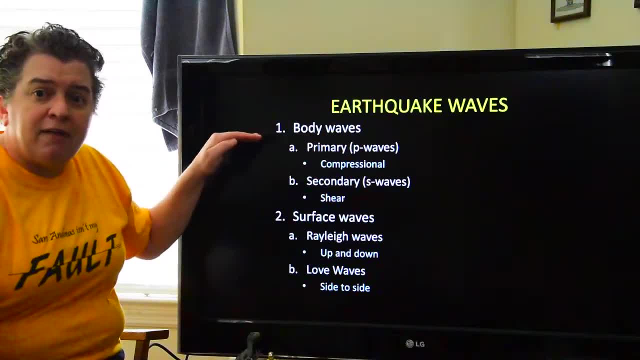 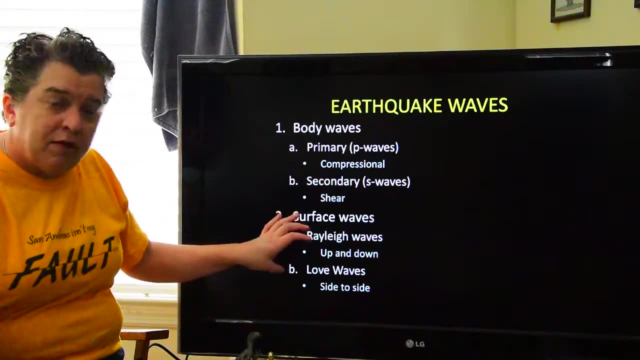 They're the ones that move the most, Because the primary waves are the fastest ones, the first ones you'll feel. Then we get the secondary waves And then the last ones that you'll feel because they travel the slowest, are the Rayleigh and. 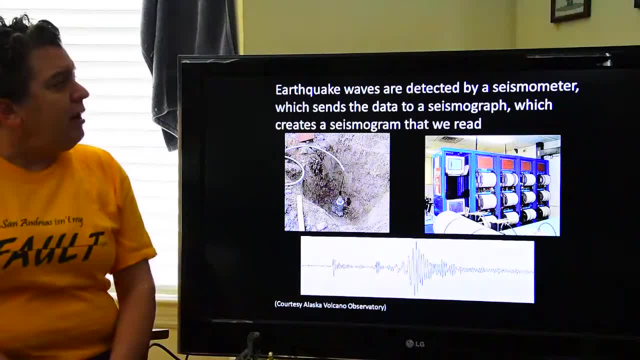 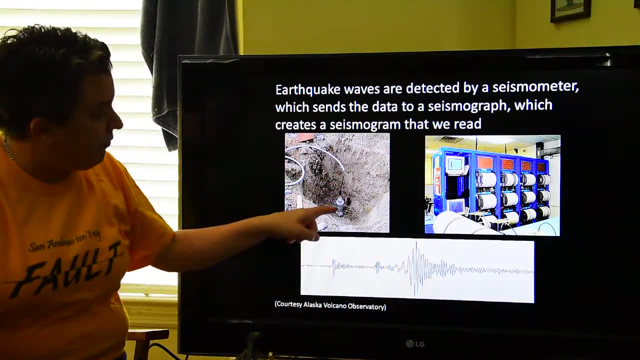 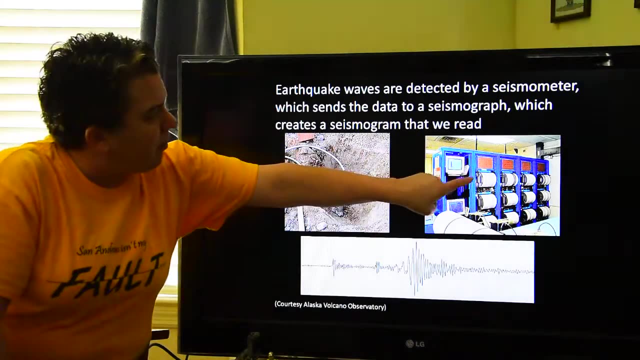 the Love waves, the surface waves, Now the earthquake waves are detected by an instrument we call a seismometer. That's a seismometer. This seismometer sends the information, the information about the shaking, to what's called a seismograph. 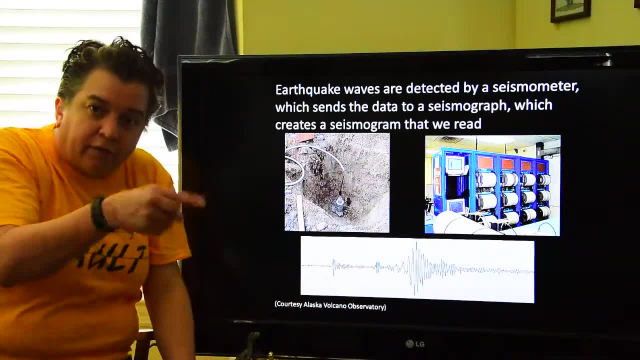 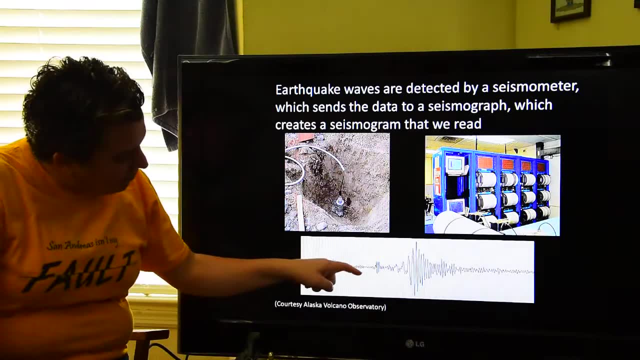 That's this thing that has the paper around it and it makes like little squiggly lines And the seismograph creates a seismogram like this: Here's the squiggly lines of an earthquake And that's what we read. 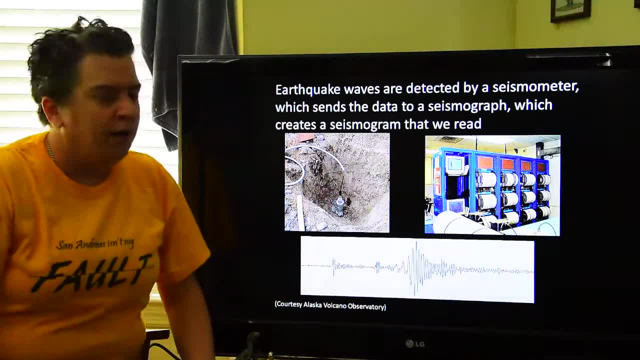 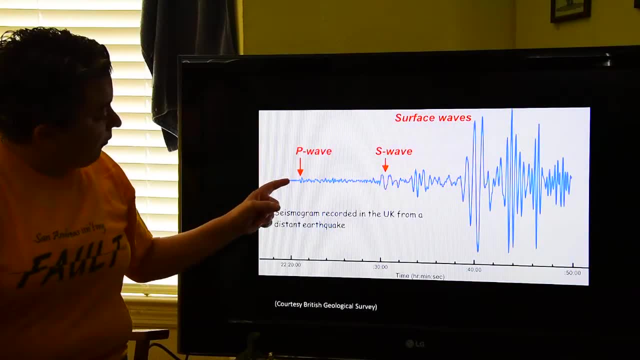 That's what I would get like on my desk and be able to say, yup, there's an earthquake. And when you look at a typical seismogram, remember I said the first waves we feel are going to be the primary waves, Then we're going to get the secondary waves. 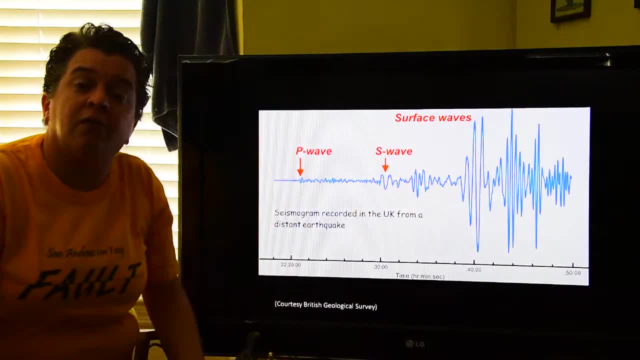 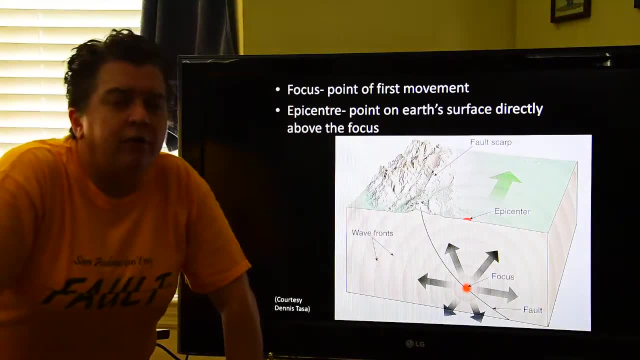 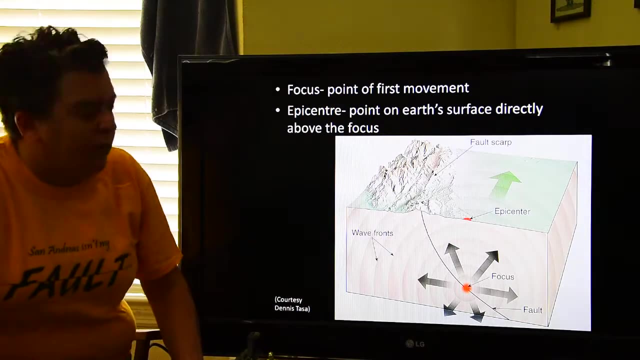 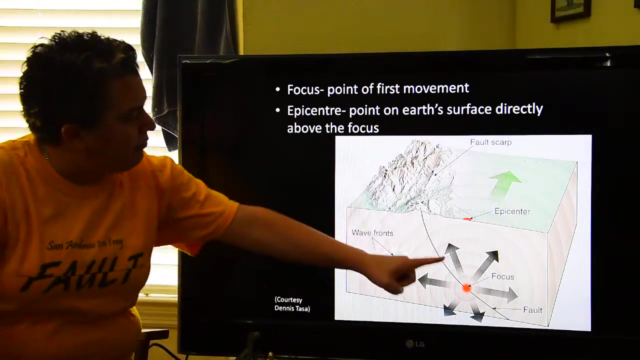 And then the surface waves arrive. What we can do with that seismogram? we can do a bunch of things like figure out where the earthquake began. So where an earthquake begins, where there's the first movement of the fault, the first release of energy, on a fault that is called the focus, a first release of energy. 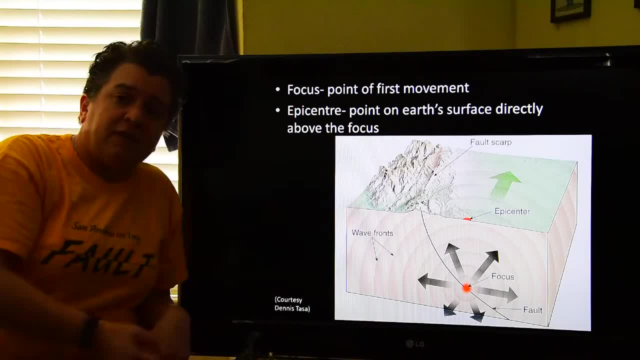 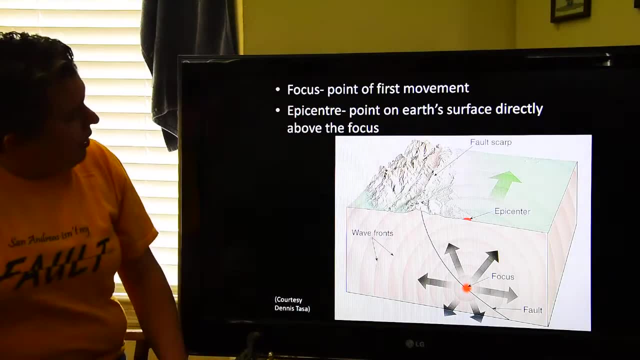 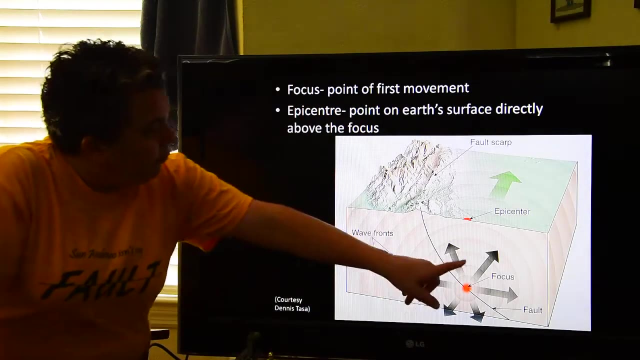 The focus can be anywhere from Earth's surface down to 660 kilometers deep, maybe even a little bit more than that sometimes. Now you probably don't usually hear on the news about the focus There. they usually report the epicenter, which is the point on Earth's surface directly above. 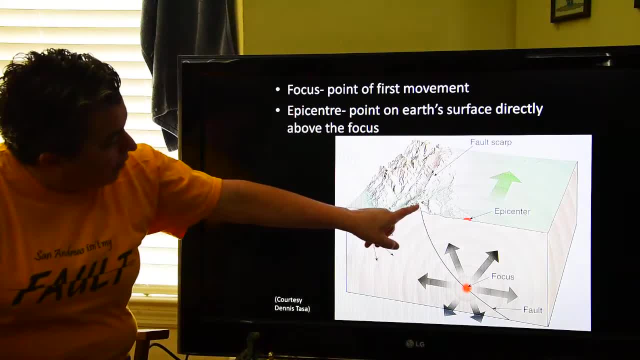 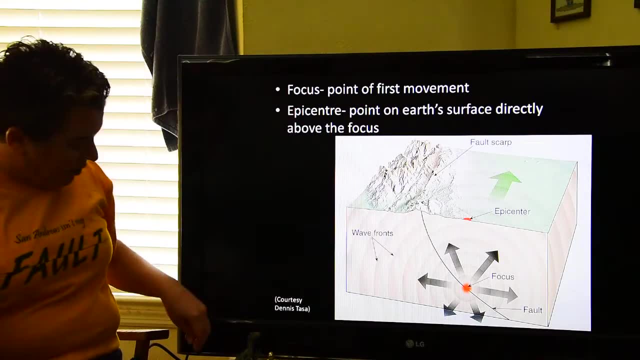 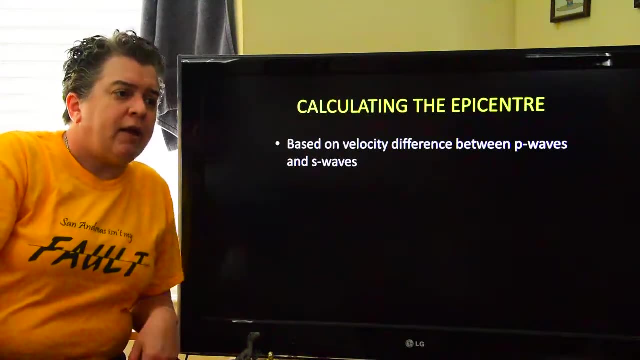 the focus, And so here we have, the fault going into the ground. There's the focus, The earthquake began, But right there is the epicenter, And when an earthquake happens, one thing that geologists have to do is figure out: where did the earthquake begin? 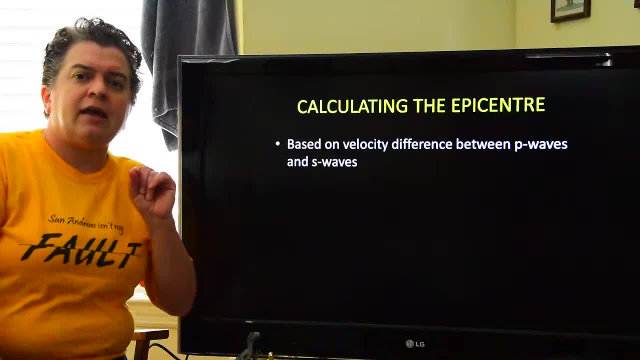 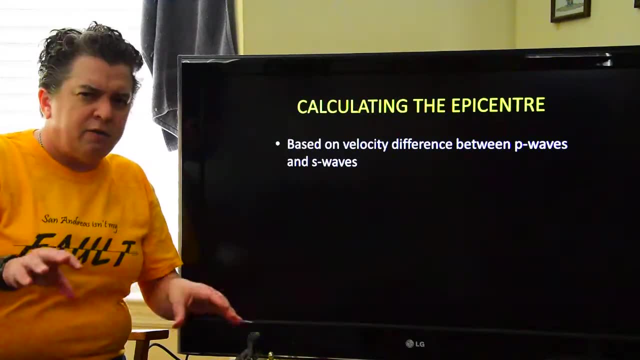 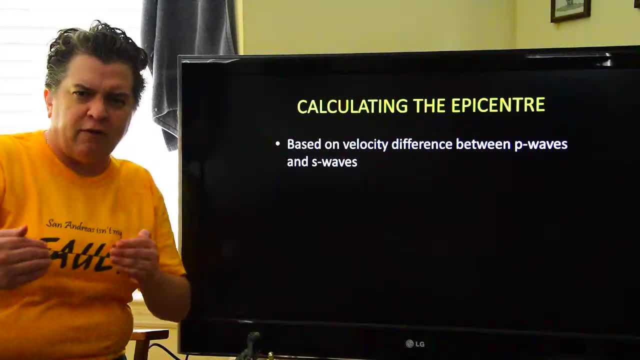 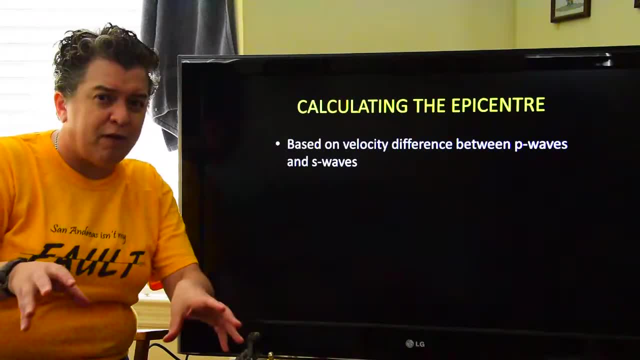 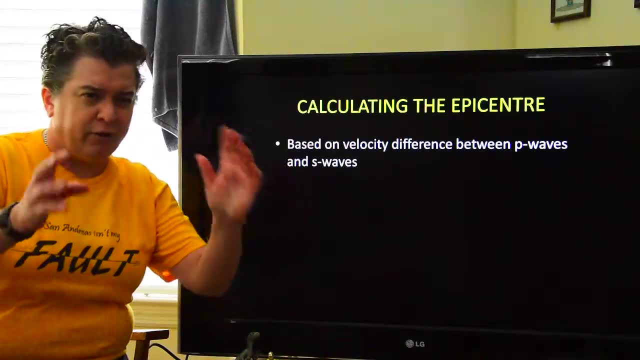 Which one arrives at grandma's house first, or something like that. You guys remember those math problems And if you're anything like me, you're sitting there like when am I ever going to have to calculate the training tables or arrival and departure times or something? 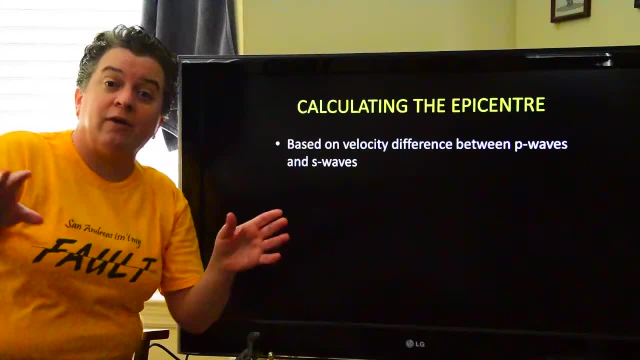 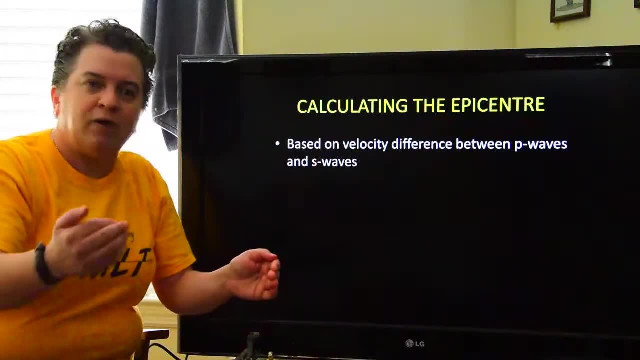 All right. Well, I'm going to tell you, Today is the day you're going to figure out why you did those problems right. So, velocity difference: right Waves are traveling at one velocity, S waves at a different. They're both leaving the point of origin. 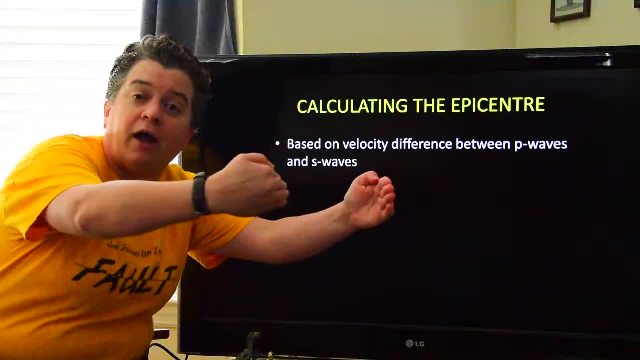 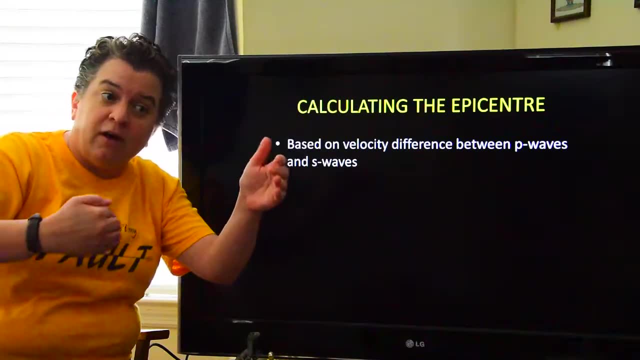 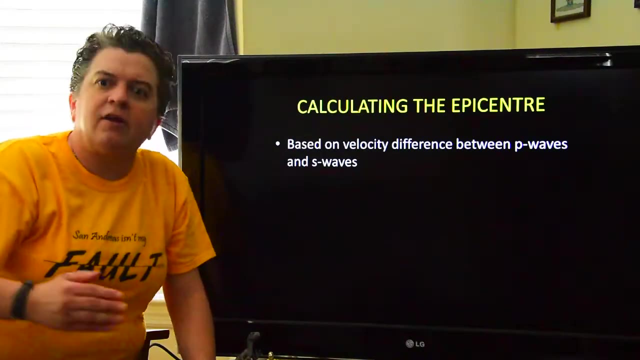 They're leaving Grand Central Station at exactly the same time. So what's going to happen then? is the time interval between both of those waves arriving where you record the earthquake? your seismograph? well, that's going to tell you how far away. 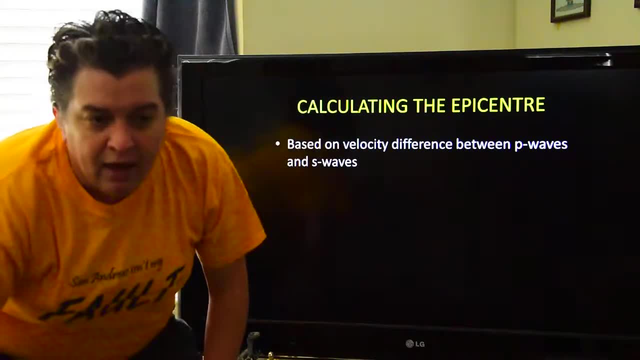 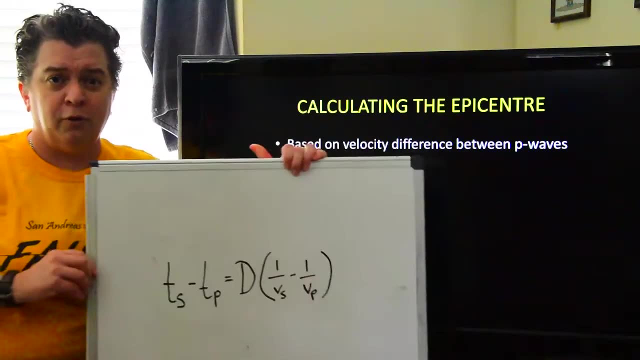 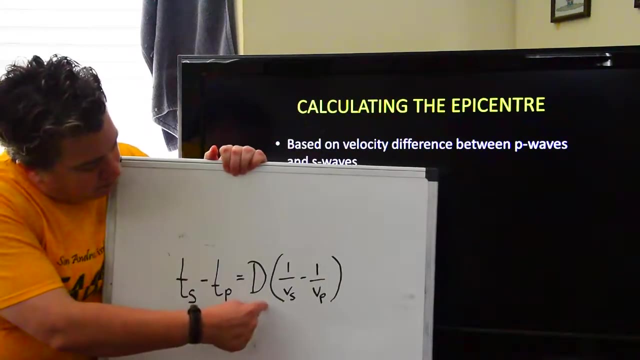 you are from the origin of that earthquake, So you can take: Take an easy equation: distance equals rate times time, and turn it into this: Doesn't quite look like the easy equation anymore, right, But we do have distance. V is rate. 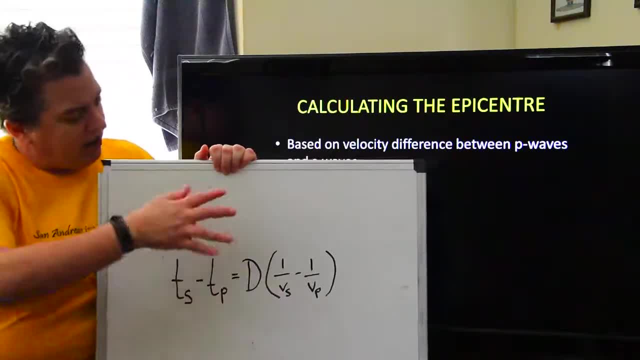 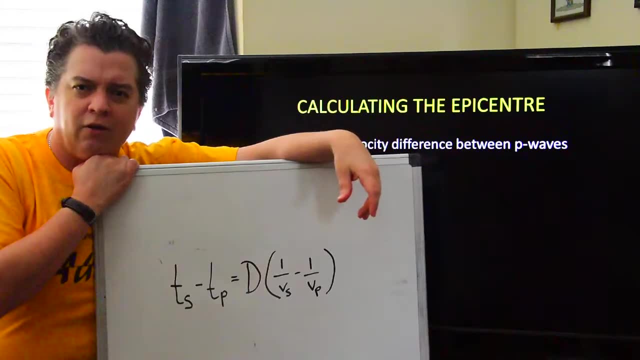 It's just velocity, T is time And I can say: from this you can calculate the distance from your seismogram to the earthquake. And you're probably going to sit there and say: but there's like no numbers, Like how do I do math without numbers? 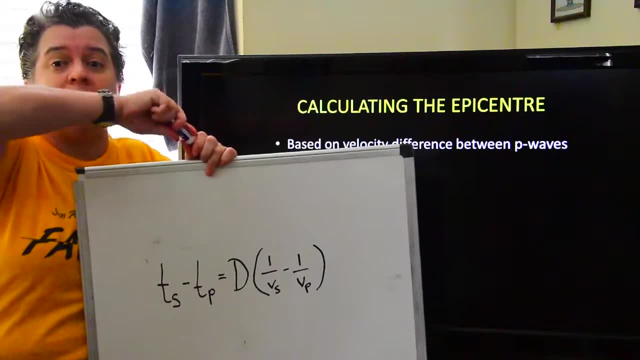 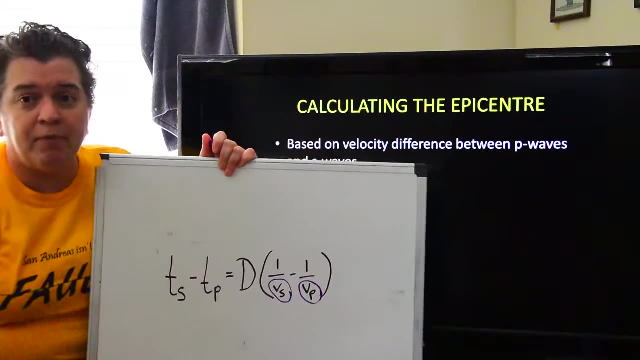 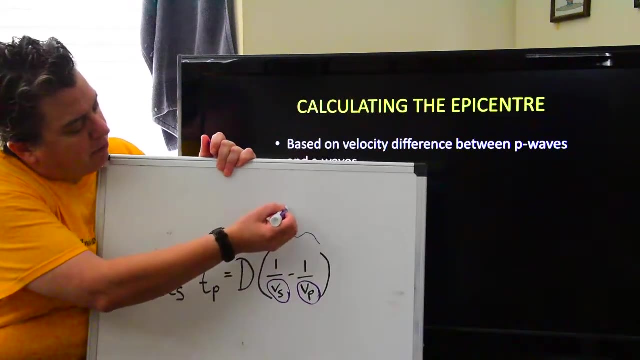 Well, it's actually not that bad. So these things- this is the velocity of the S wave and the velocity of the P wave, And those are constants, So this becomes a constant. It's really hard for me to write like this. 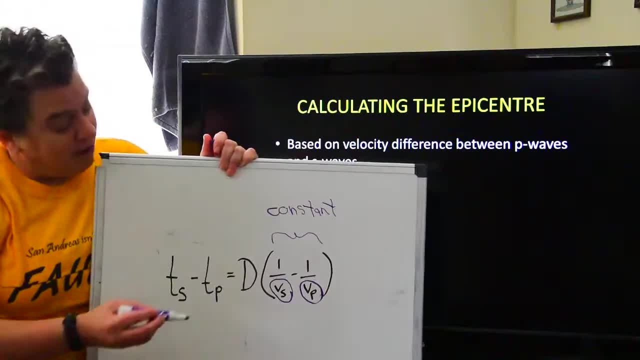 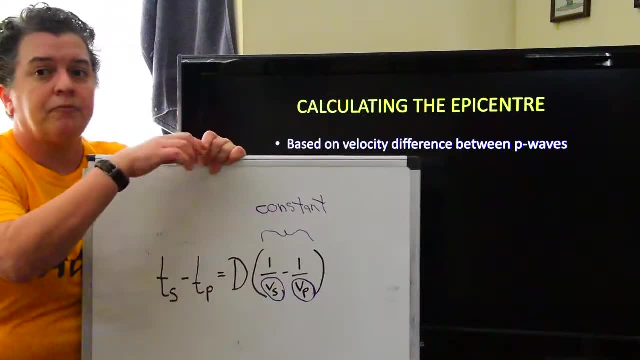 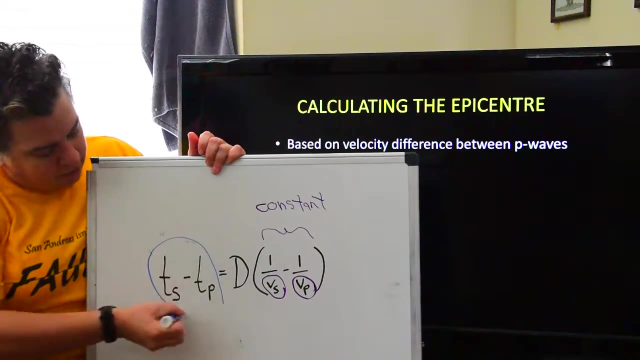 So it looks like I'm in kindergarten. So that's a constant. A constant is an unchanging number, So this becomes a number. All right, That's good, We got rid of some of those letters. Well, what about this thing right here? 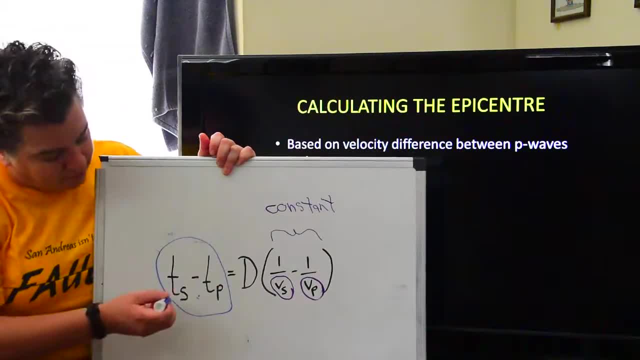 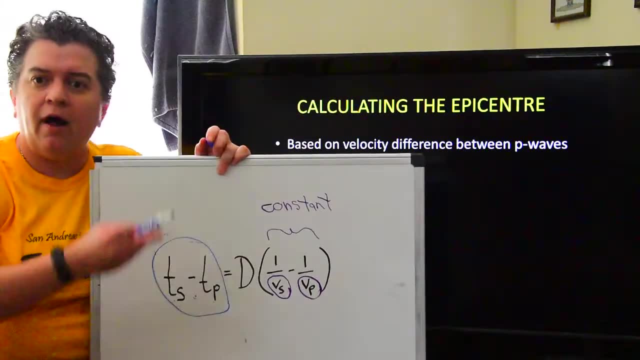 This gets measured from the seismogram. That's the time the S wave arrives and the time the P wave arrives, So that's going to be a number as well. That's going to be like 28 seconds or three seconds or something like that. 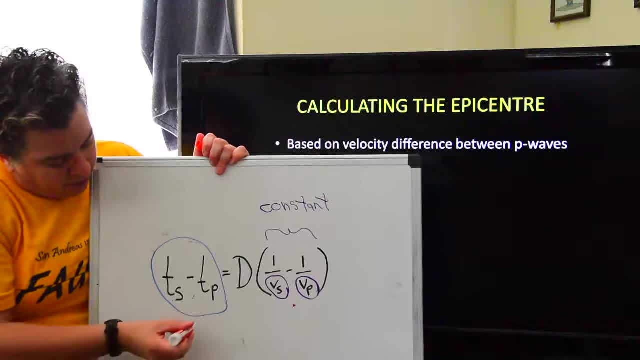 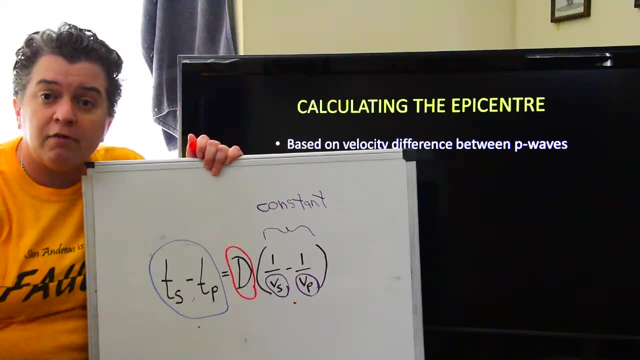 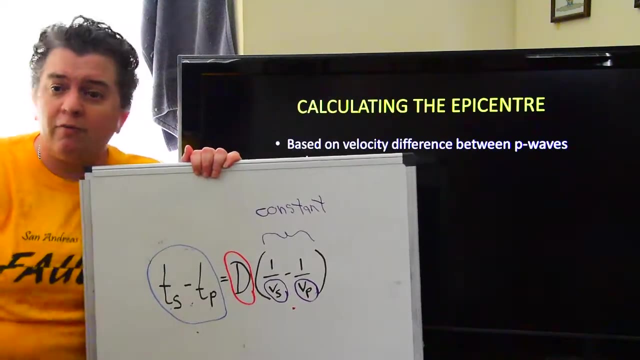 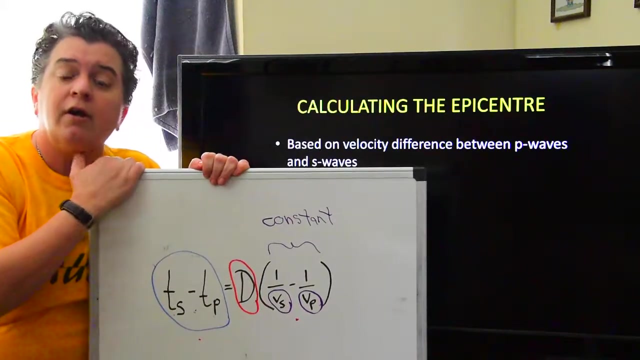 So now We have a number over here, a number over here and a single variable, d, which stands for distance. So just by using the velocity that the P wave and the S wave travel at and the time interval between their arrivals, you can calculate the epicenter. 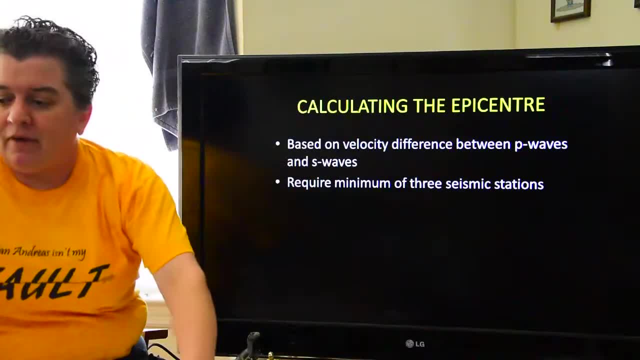 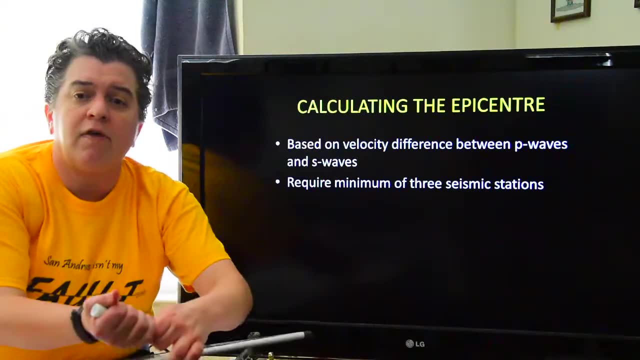 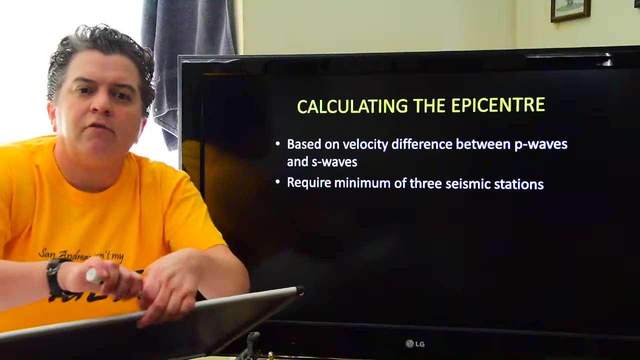 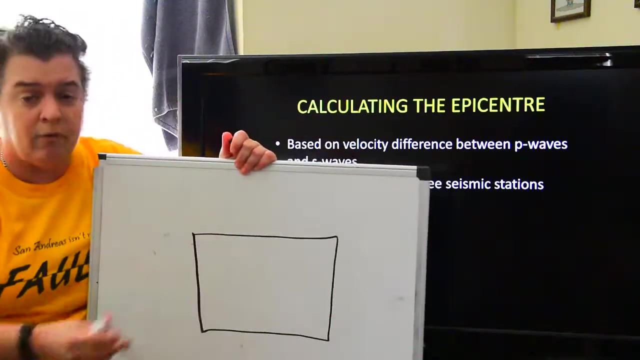 However. So Okay, So You need a minimum of three seismic stations to do that, because that handy equation that I just used just tells you distance, right? So let's imagine I'm in Colorado because I suck at drawing and Colorado is a like rectangle. 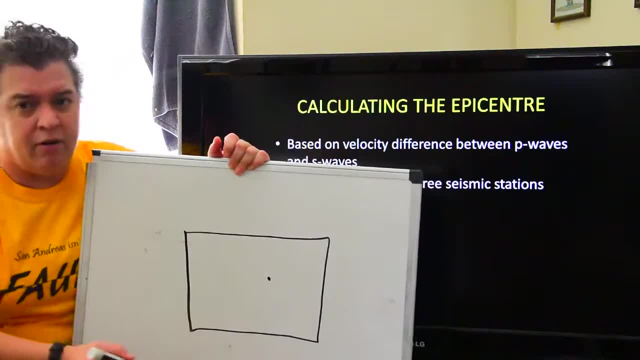 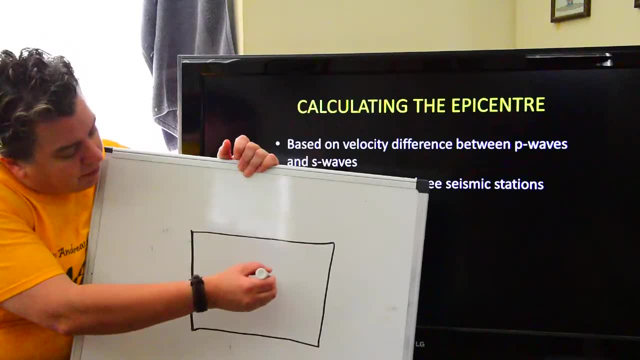 right. So let's say we're in golden Colorado- Good reason to be there. There's a brewery there too. So anyway, let's say we have a seismograph there that records an earthquake, That's like I don't know, 150 kilometers away. 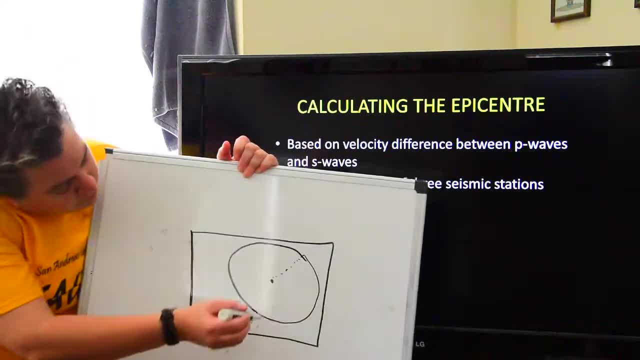 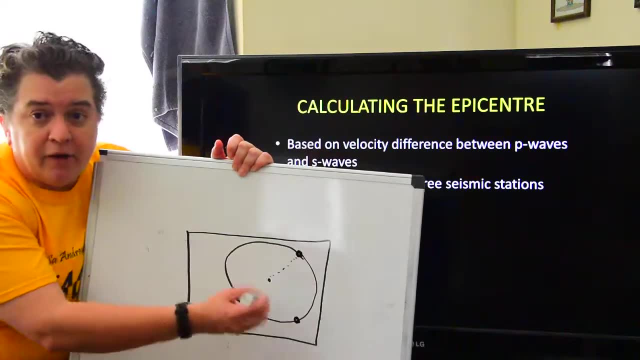 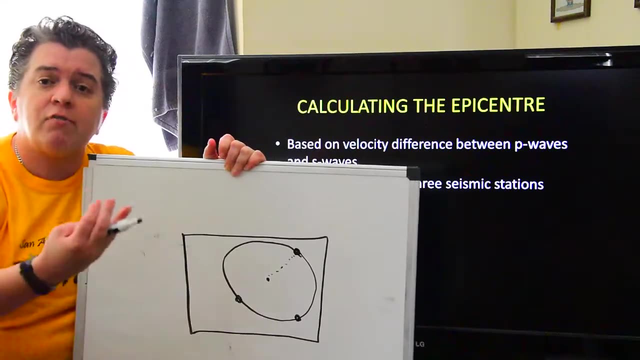 Well, I only know it's 150 kilometers away. I don't know if it came from up here or over here or over here, I just know the distance. And so the reason we need three recording stations is we have to do something called. 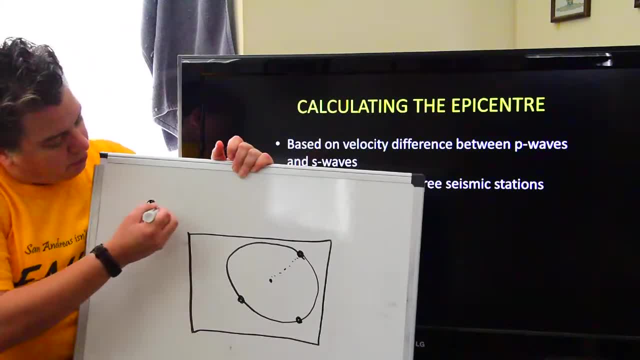 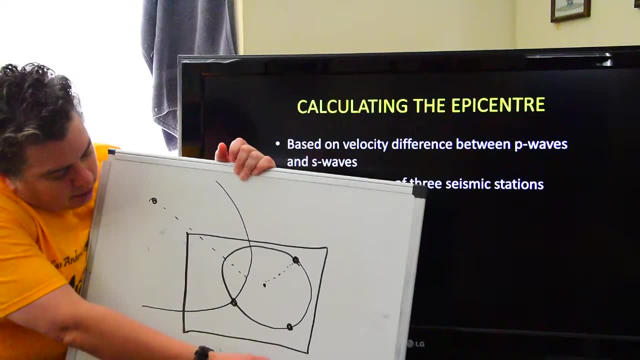 triangulating. Maybe the guys up here in Utah are like, Oh, we got it at being like 400 kilometers away, And the guys down in New Mexico are like, yeah, and we got it at being I don't know however far away that is. 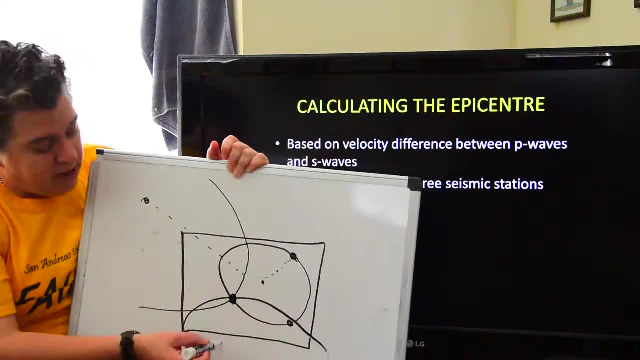 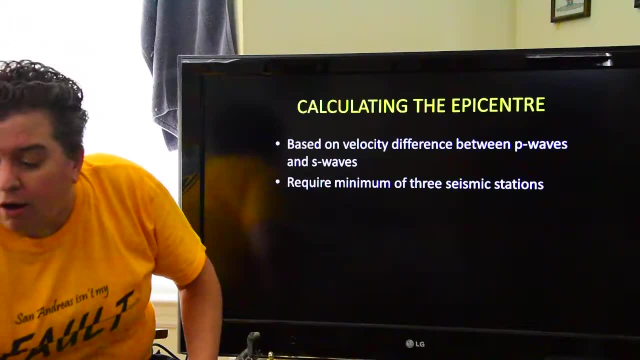 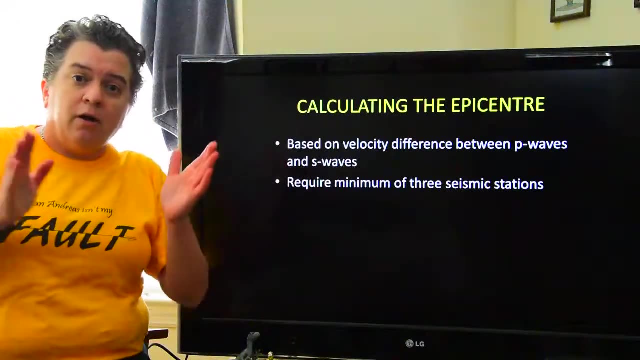 And so we're all three of those circles meet. that tells us that's where the epicenter is. So just remember, if you are recording the or figuring out the epicenter of an earthquake, you look at the arrival time of the P and the S waves. that tells you the distance you.